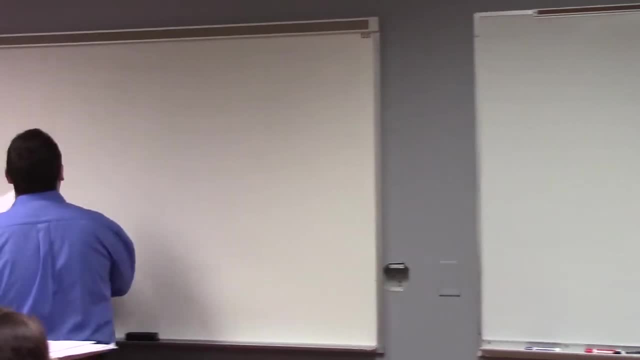 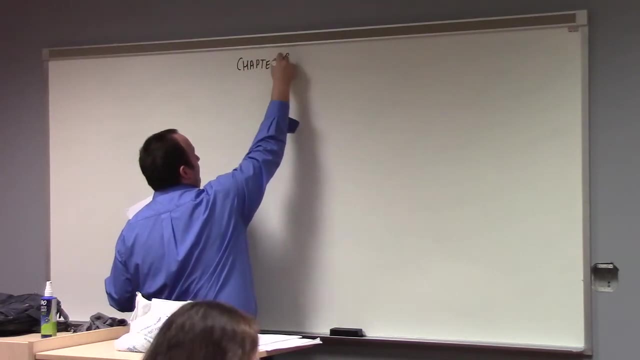 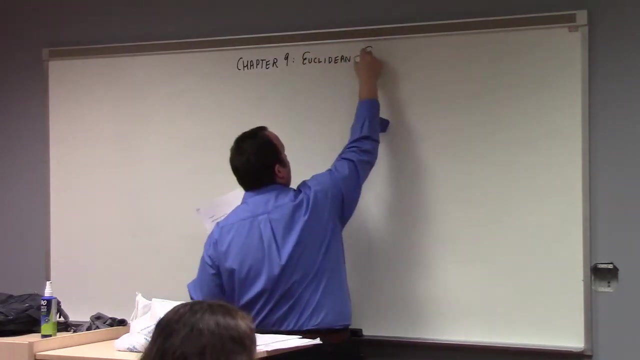 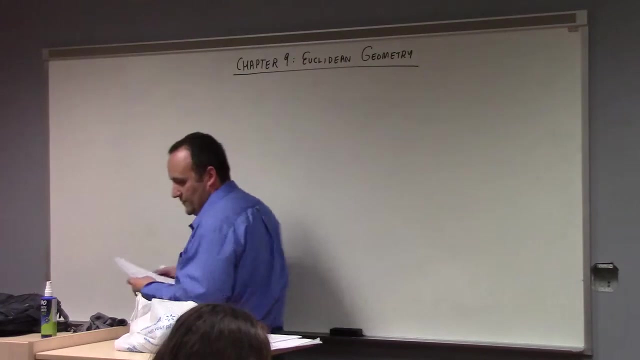 All right, so we are now into chapter 9, and chapter 9 is on Euclidean geometry. So up until now I sort of dodged the question for the most part about angles, Angles, Lengths And many of the geometric questions you might ask. 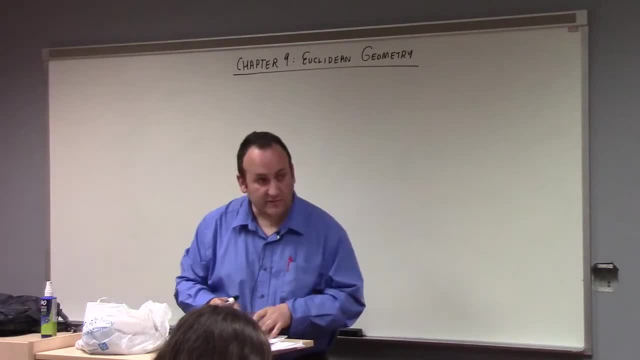 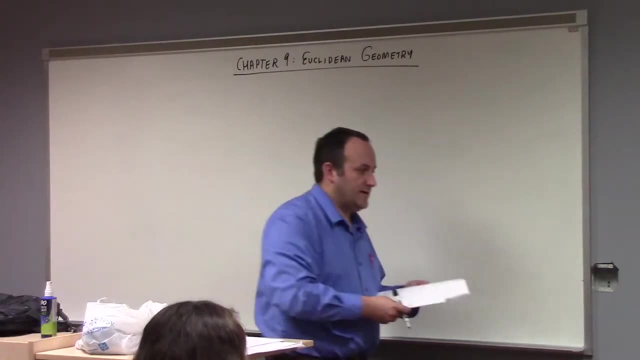 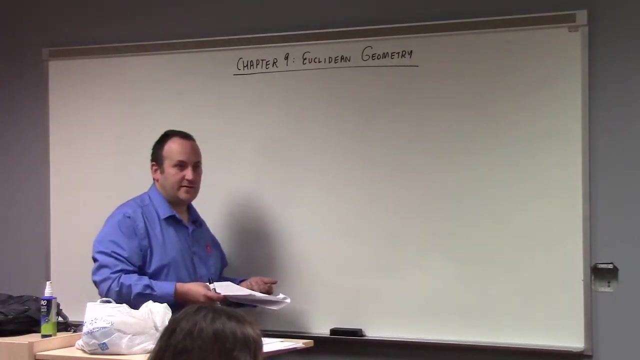 So today I'm going to define a couple of notions, in particular the inner product and also the norm of a vector, And with these concepts we can talk about the length of a vector or the angle between two vectors, generalize the notion of perpendicularity or two vectors being perpendicular. 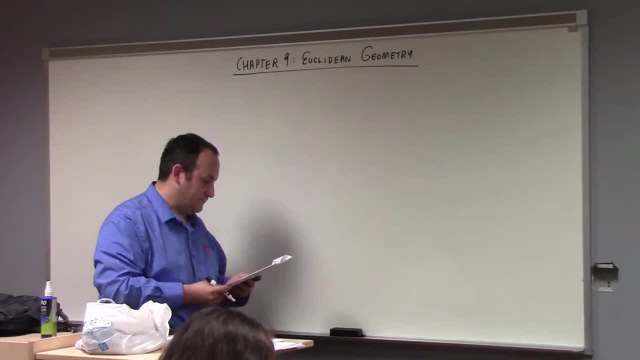 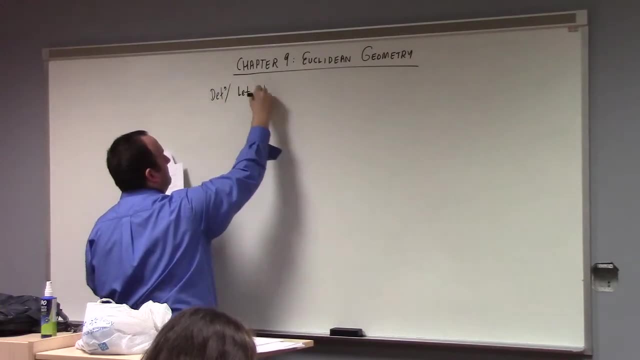 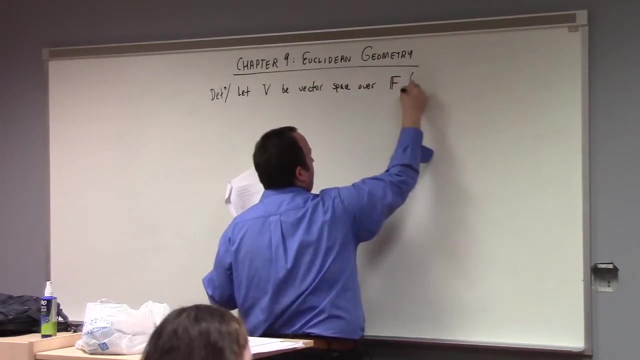 We say they're orthogonal in here. All right, these are things we'll do. Let me get started. So let's get right into it. So there's the definition. Let V be a vector space over F, And this is either going to be R or C. 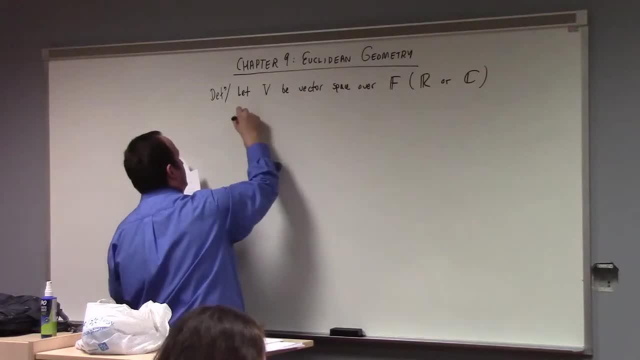 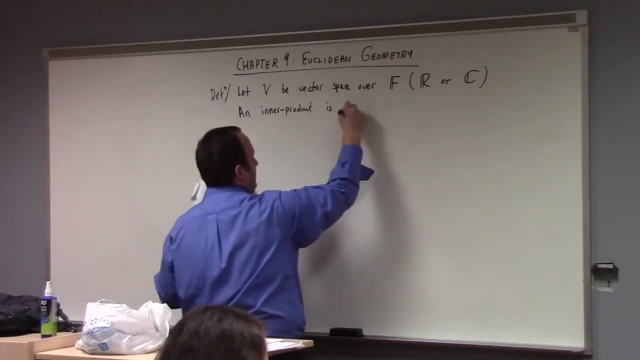 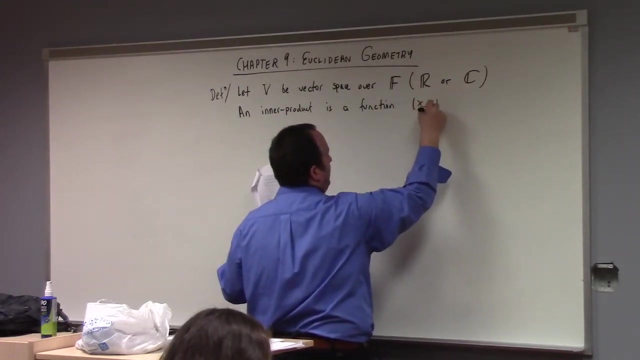 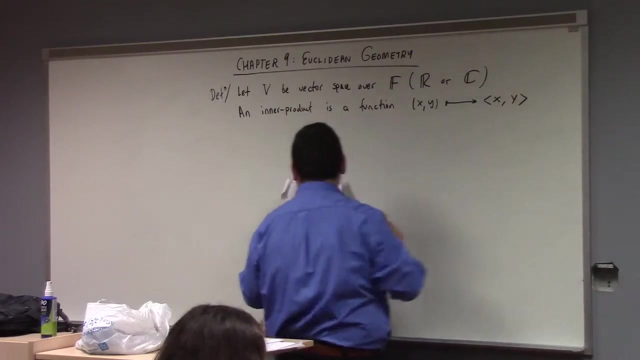 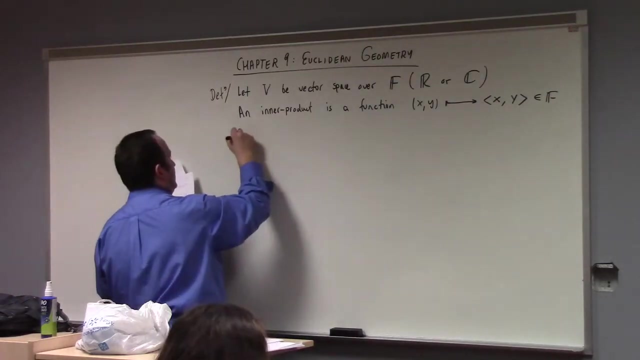 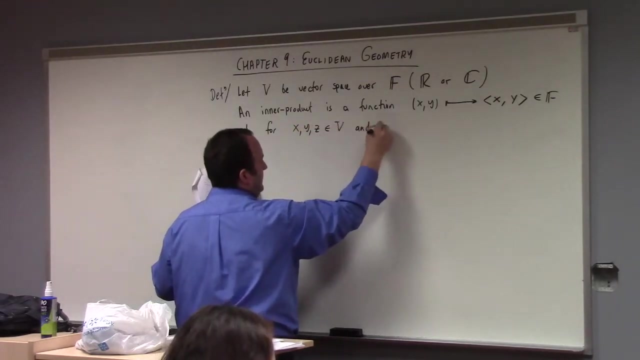 All right, Then an inner product is a function, All right. That say, takes X, comma, Y and maps it to X, lingle X, Y, wrangle an element of F, all right, such that for X, Y and Z in your vector space and scalar C, we have the following: 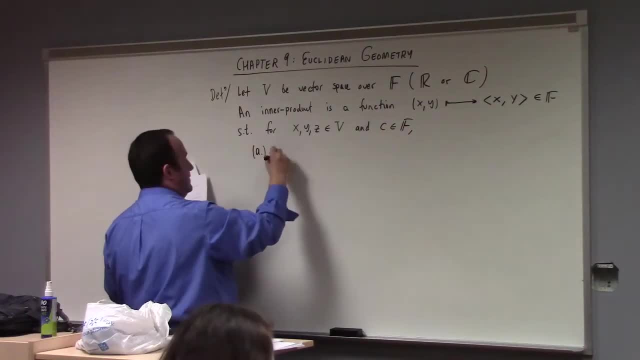 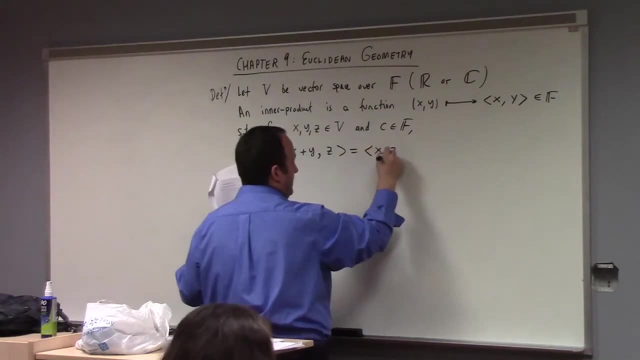 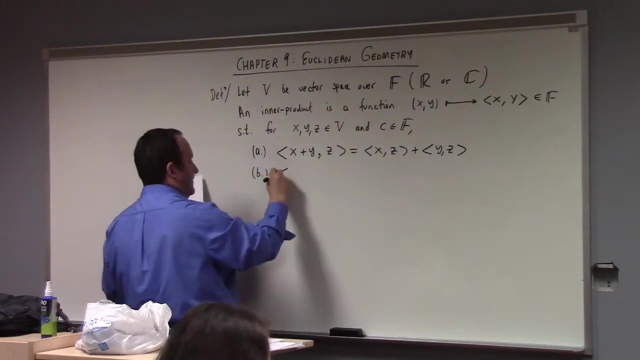 We have the following. We have the following: A- we have additivity in the first slot, X plus Y. comma Z is equal to the inner product of X with Z plus the inner product of Y with Z. Part B: we have, in fact, the ability to pull a scalar out of the first component. 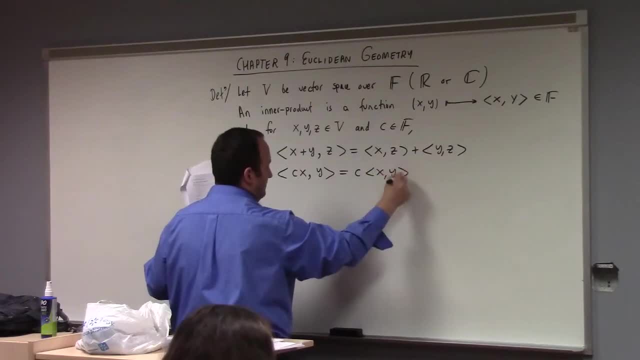 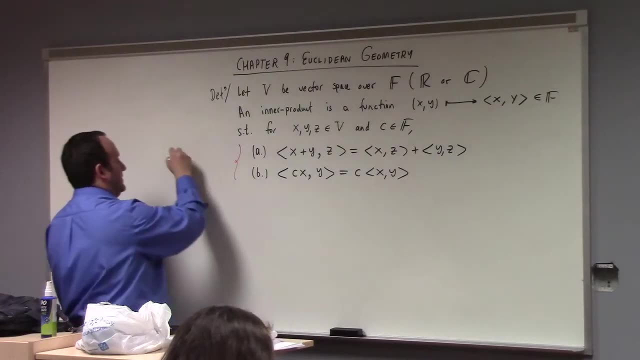 Inner product of C, X with Y is C times the inner product of X and Y. So, taken collectively, items one and two I would refer to as linearity in the first slot of the inner product. All right, This is what A and B give us collectively. 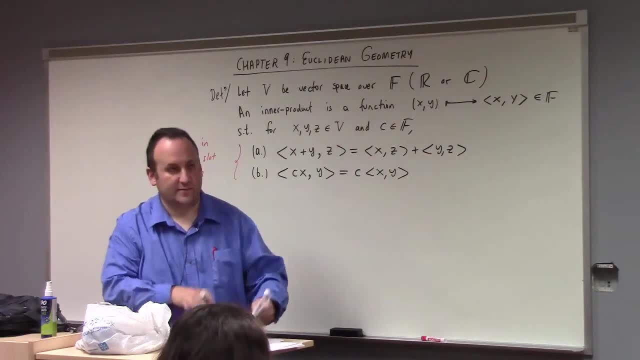 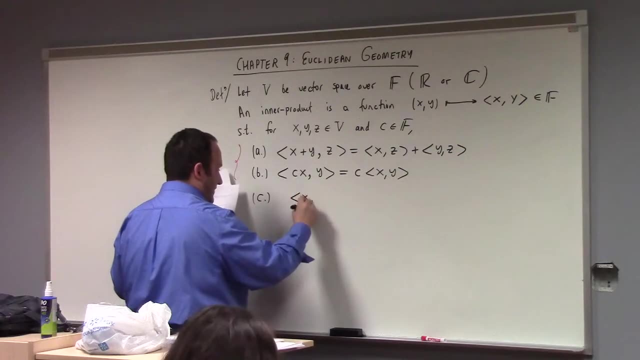 However, we don't have linearity in the second entry. generally speaking, In the complex case at least, it's not the case. So what we do have for axiom C is that the complex conjugate of X and Y is equal to YX. 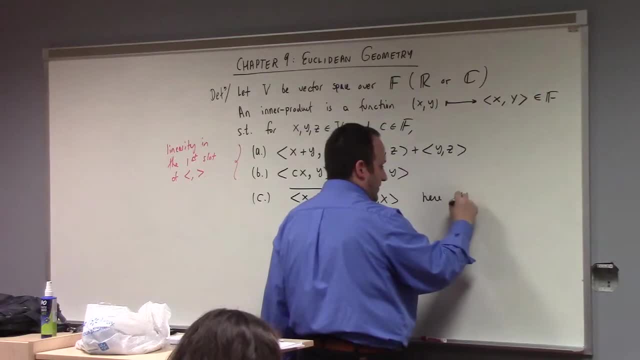 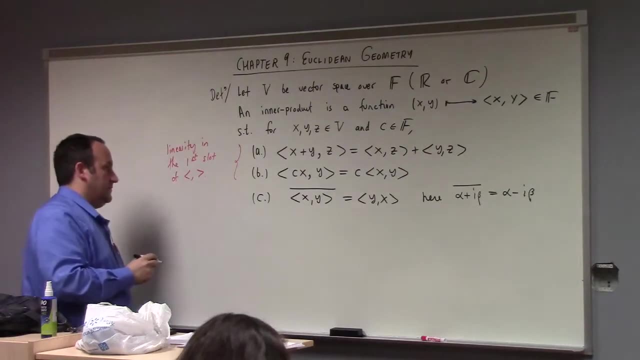 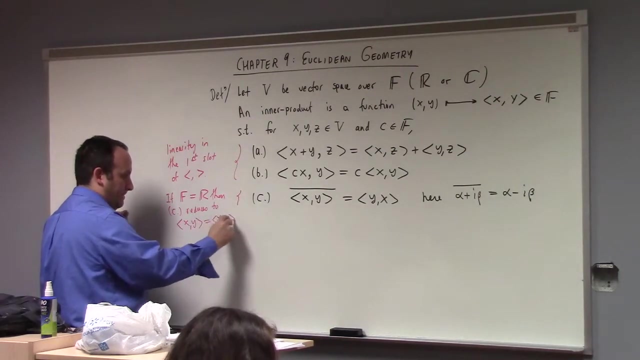 Here, like alpha plus I beta, conjugate is alpha minus I beta, right, And you know side comment. So if our field is the reals, then C reduces to what. So, in the case of, we're working with a real vector space and a real inner product. 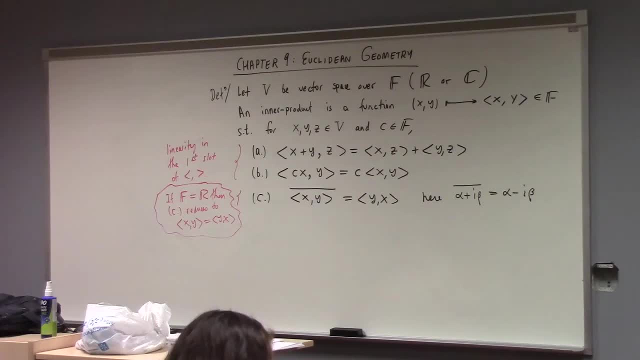 part C of the definition just says that the real inner product has to be symmetric, That it doesn't matter if you do X inner product Y or Y inner product X. the answer is the same: Symmetric, Symmetric. Why do we not say it can be a real? 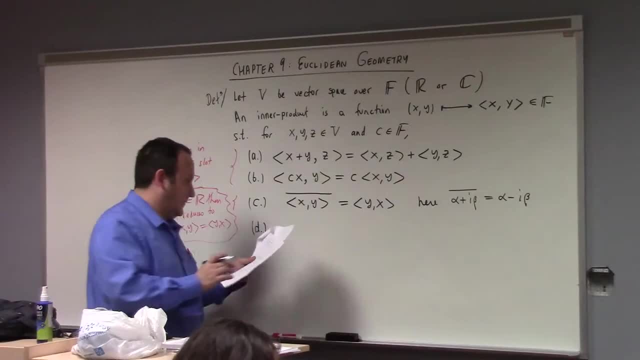 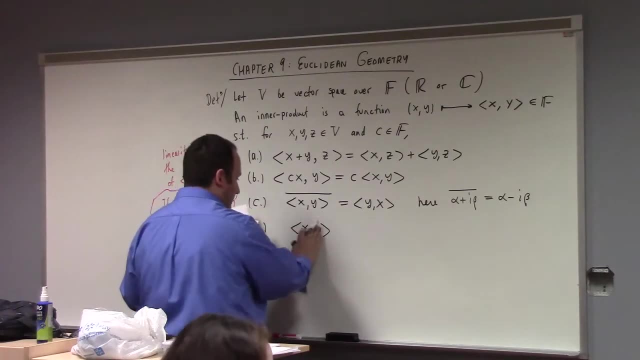 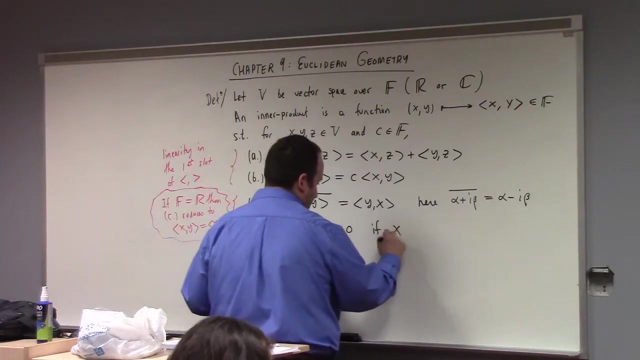 You could say commutative, but we usually say symmetric, And then I mean we certainly would say that the dot product is commutative. That's a typical oops. you got me. Inner product of X and X is greater than zero if X is not equal to zero. 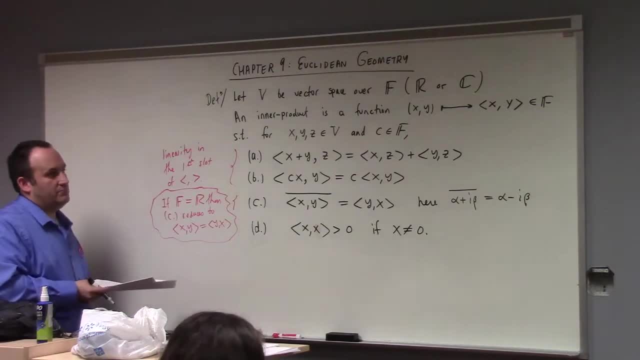 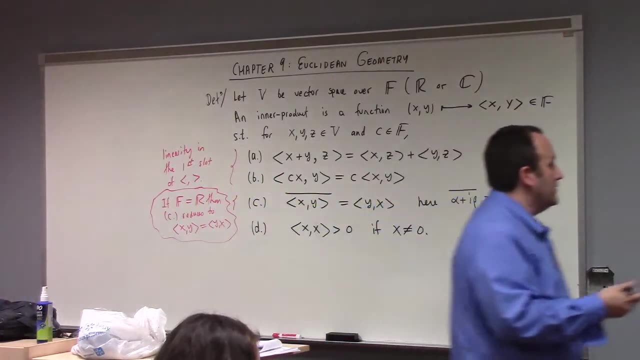 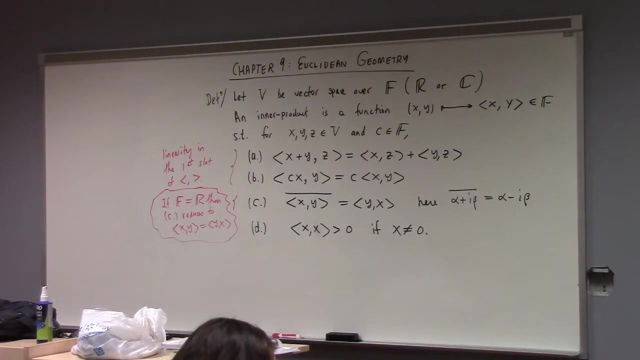 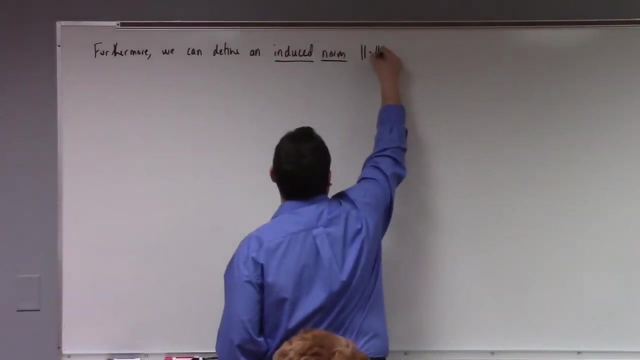 All right, So this is an inner product. Now, what's the What's the purpose here? Well, furthermore, we can define an induced norm, which we use this notation for. So this is a mapping from the vector space. 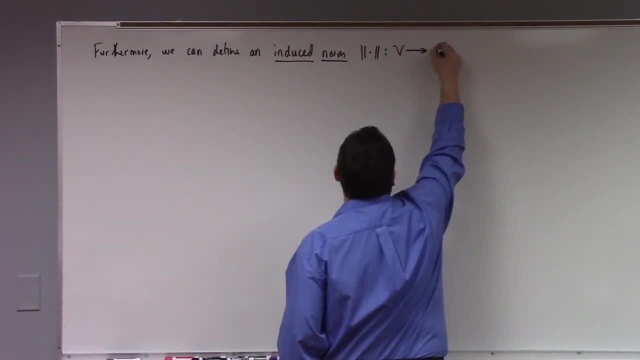 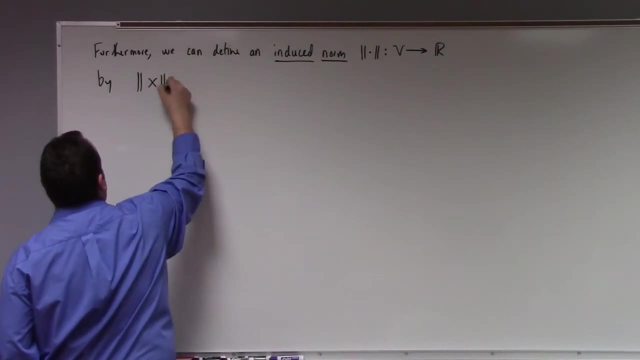 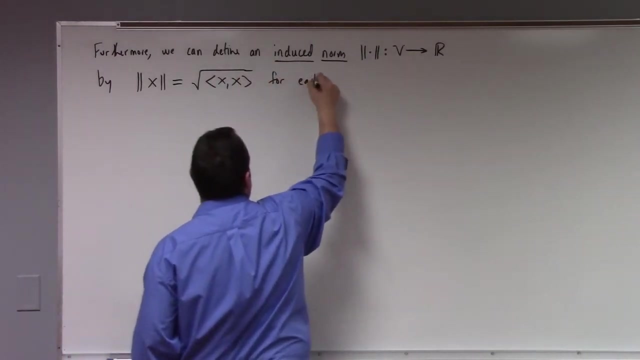 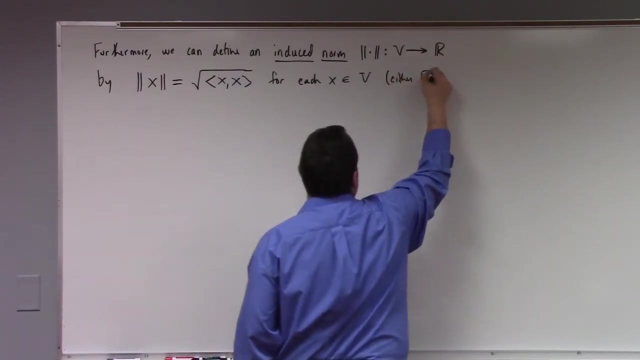 to the reals By here it is. The norm of X is equal to the square root of the inner product of X and X. X in V, And this is either F equals to R or C. So this is the so-called induced norm. 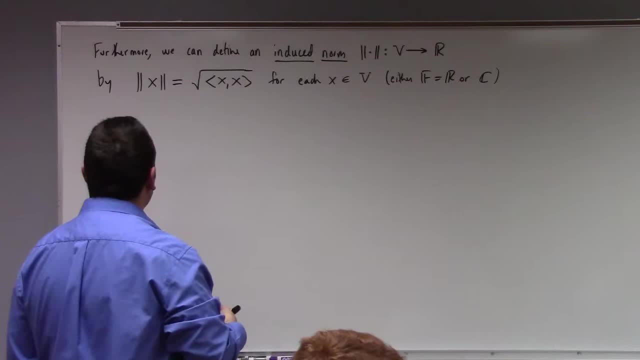 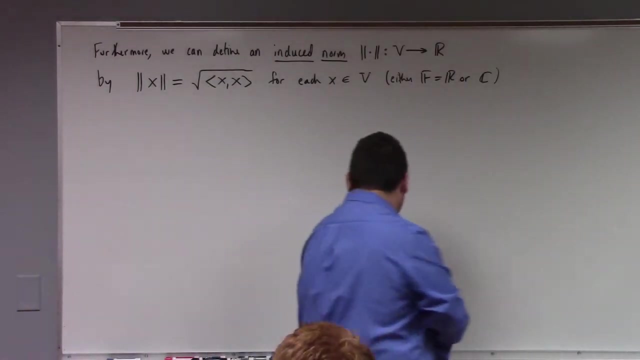 What is it? I'm happy to explain. I just couldn't read all the way over there. Oh, I'm sorry. Sorry, I could do it once. All right, Sorry about that, And I've used the worst color possible to do that. 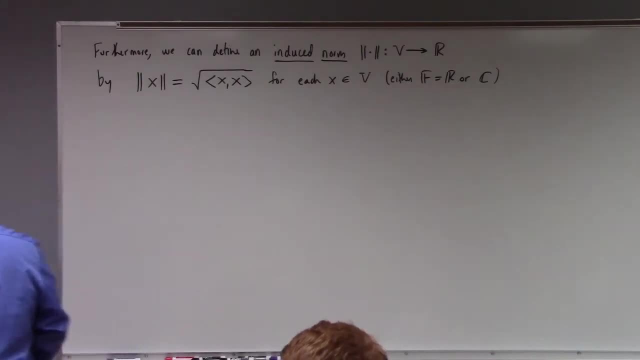 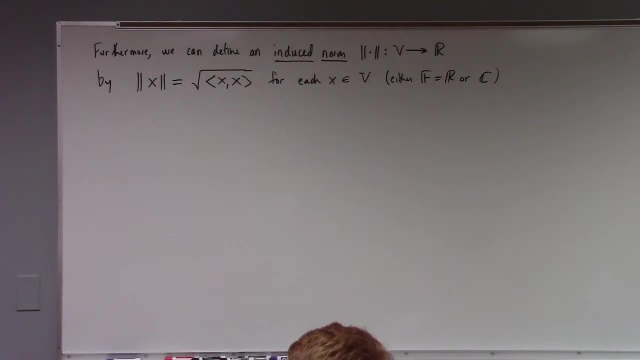 By the way, an inner product, a vector space paired with an inner product, is called a quote-unquote inner product space. So you could say V comma lingo wringo is inner product space. What's that word you're using for what? 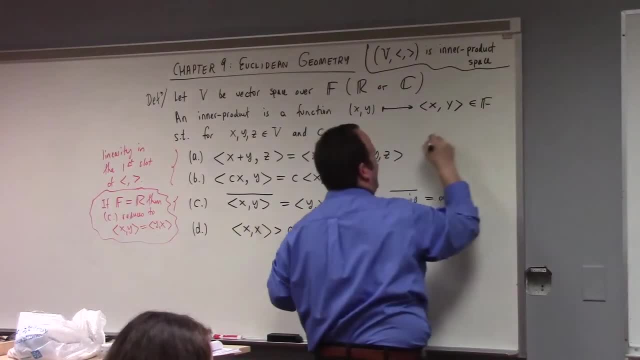 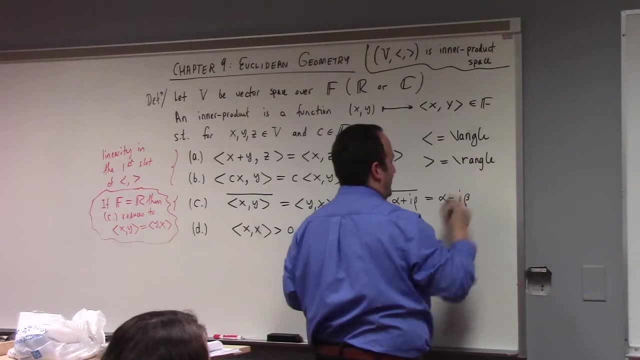 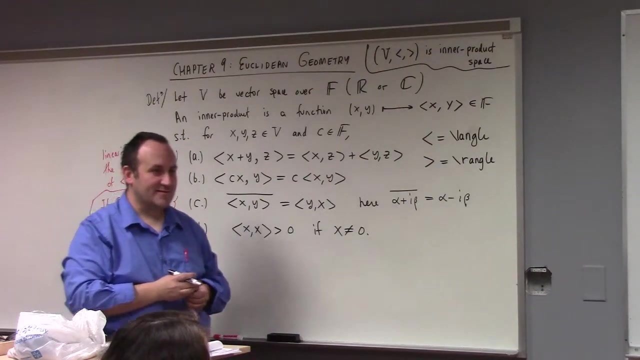 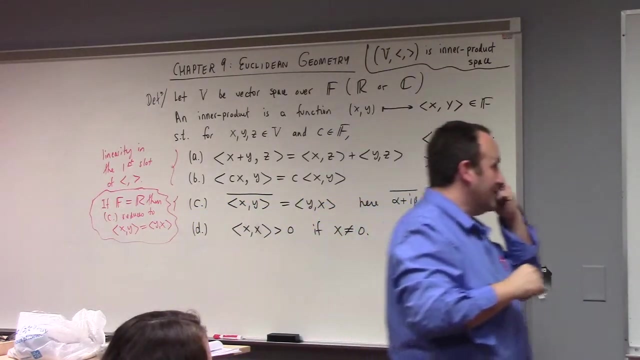 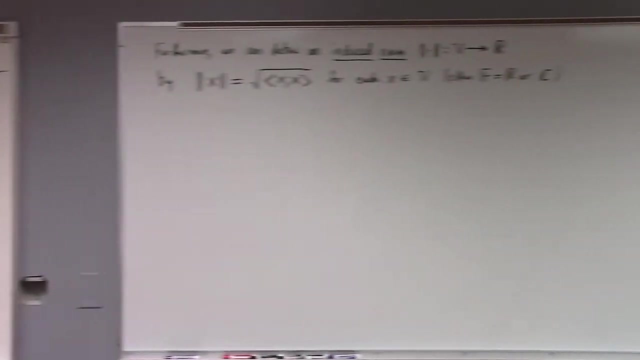 So this symbol in tech is left angle And this symbol is right angle. So I refer to them affectionately as langle wrangle because that's their LaTeX. But I just mean bracket angle, bracket. Sorry, They're not the same as like less than or greater than. 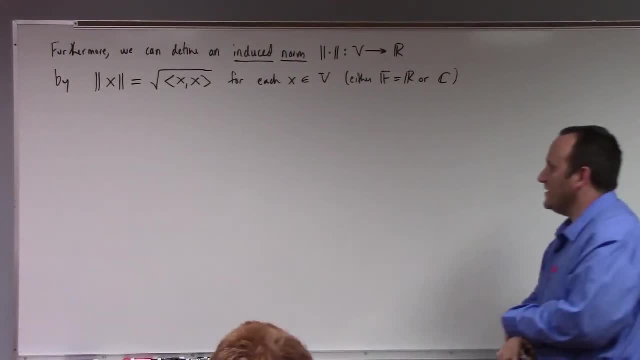 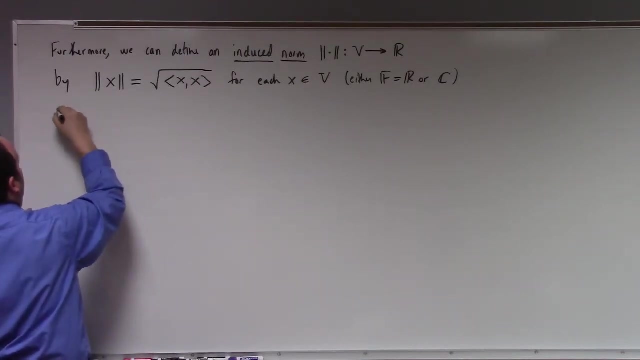 Those are more. they're different Now. so a vector space paired with an inner product is an inner product space. A vector space paired with a norm is called a normed linear space, And we can prove that, in fact, the norm of 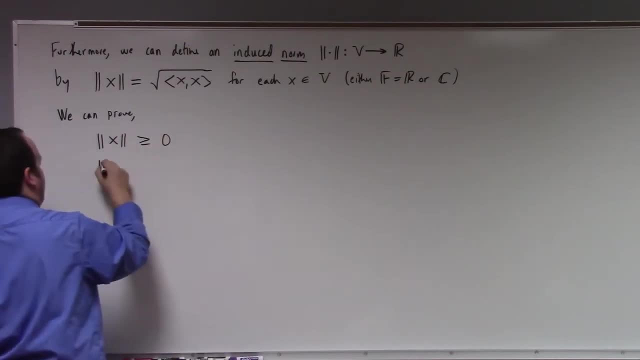 of course, the norm of x is greater than or equal to 0.. We have that the norm of x plus y is less than or equal to the norm of x plus the norm of y. We have that the norm of a constant times x. 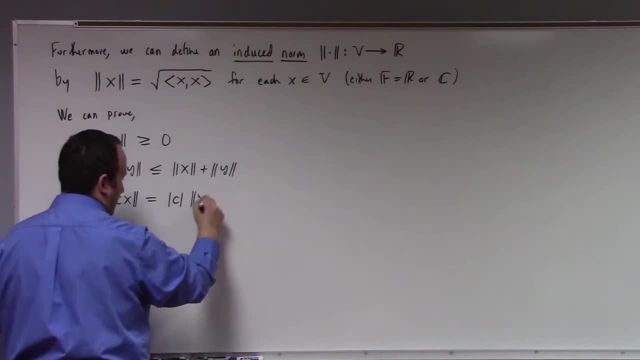 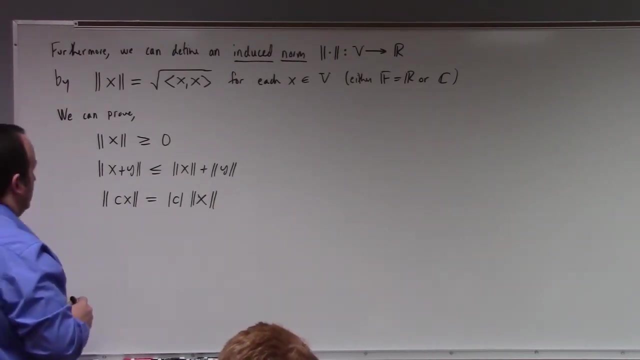 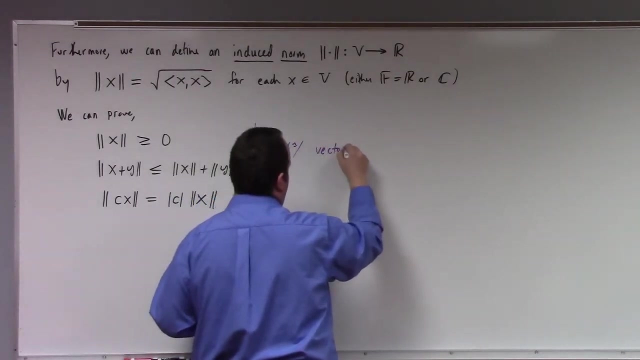 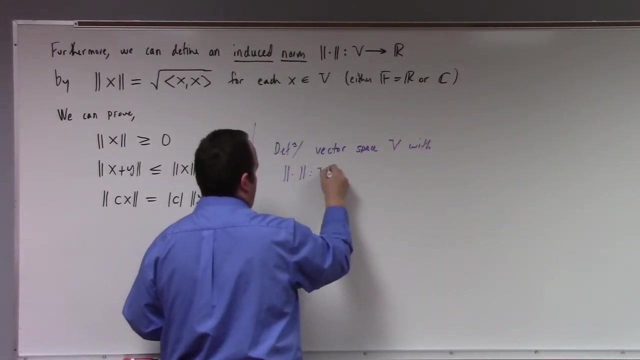 is equal to the absolute value of the constant times, the norm of x. These, these things are all true for the induced norm. all right, these things are all true for the induced norm, and indeed so, in addition. so I just you know. definition: vector space V with a function double bar, like, denoted, like. 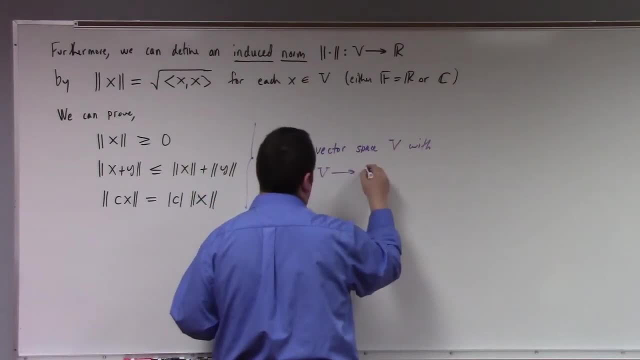 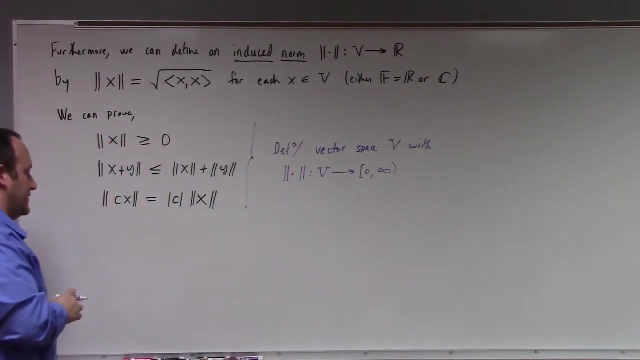 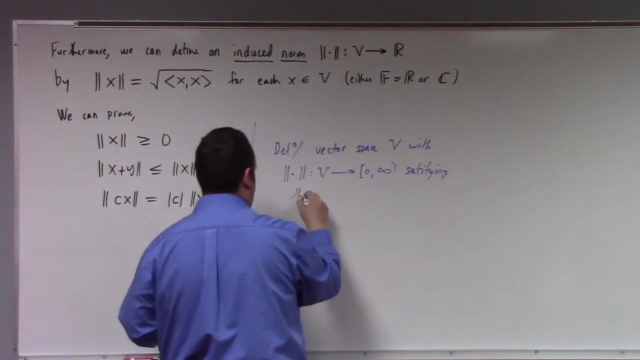 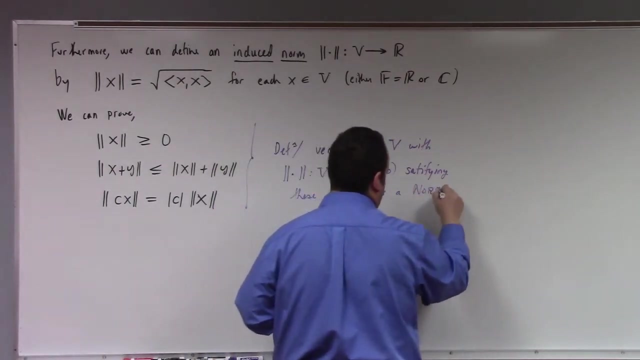 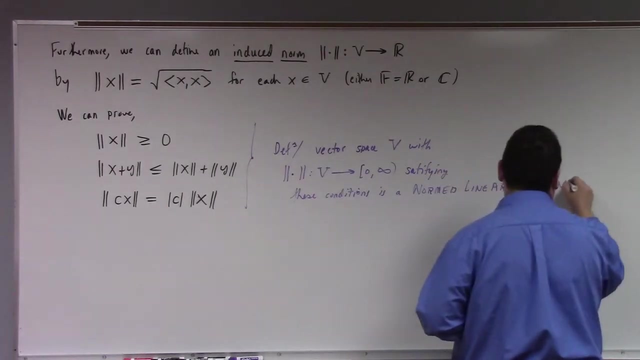 this, that takes V from to the to the positive, positive, non-negative real numbers. satisfying you these conditions is a normed linear space, which, of course, you might call an NLS. this is a normed linear space. so what I'm claiming at the start of all, 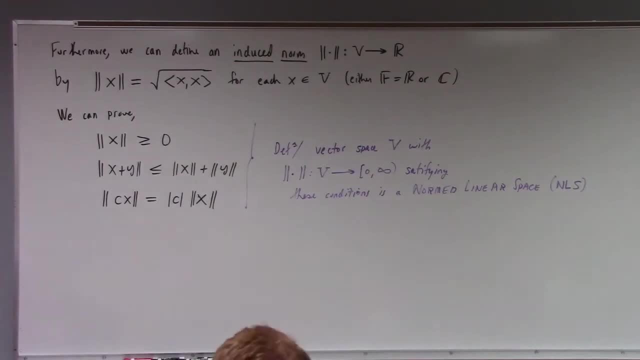 this is that if you have an inner product space, you can build a norm from it, the induced norm, and so any inner product space is also a normed linear space with respect to this norm. that's kind of nice, but it's more than that. you also have this Cauchy Schwartz inequality, so this is an in addition. 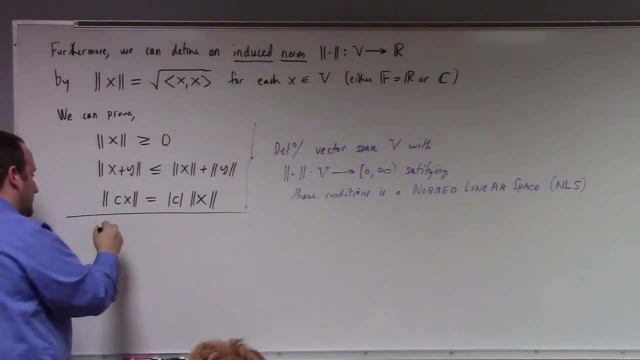 this is just this together just defines a normed linear space. we also, in the case that the norm is induced, have this, this nice relation, the- I shouldn't write, I should say the absolute value, and again it's all tubes, yeah, and also by everyone suggesting it with multiple curves, it doesn't mean you. 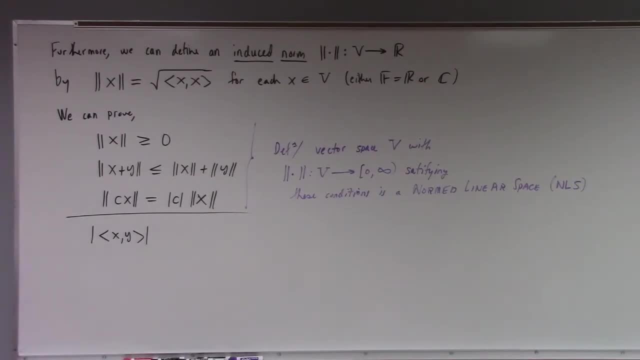 can use just the minimum or you don't want to do. look at this. just ask for a word of the what I'm. what doeshabon draw is one know the hash bar for the 북한 real number that's going to be, or between this one in, you can really. 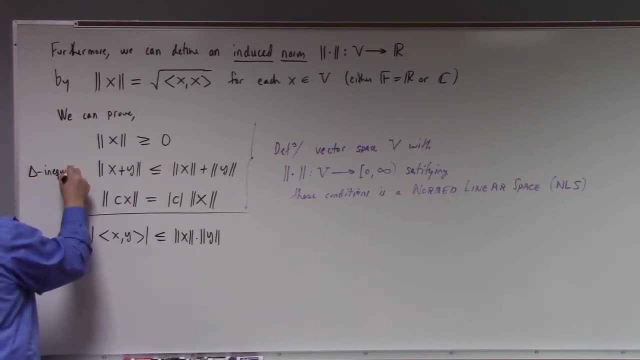 좋을 and third-party models to convert to表 did not not this, but the the absolute value right. so this is either the absolute value in This. down here is the Cauchy-Schwartz Inequality. Now I have proofs for the Cauchy-Schwartz Inequality and the Triangle Inequality, both on page 260 of the notes. 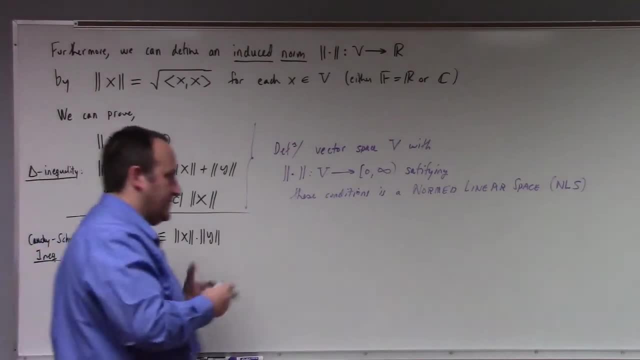 I want to focus most of our attention here on class, on examples, so I'm going to avoid the temptation to prove those in here, But I wanted to put this out in front of us. like in the past, I've defined inner product space. 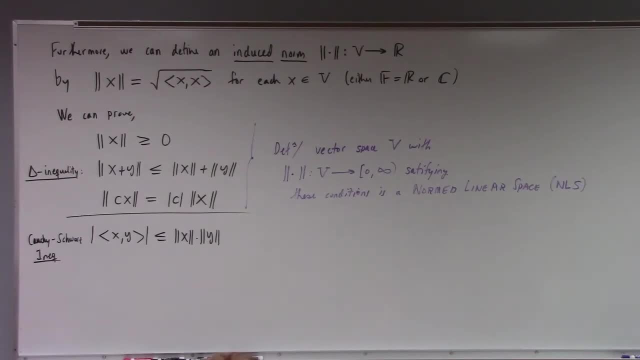 and then talked about it for like 20 minutes, then talked about the norm. But I think it might be helpful to define them both at the start so we can look at both the inner product and the norm. for my examples like parallel: 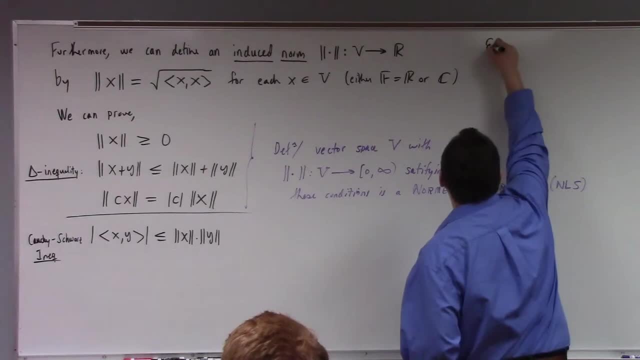 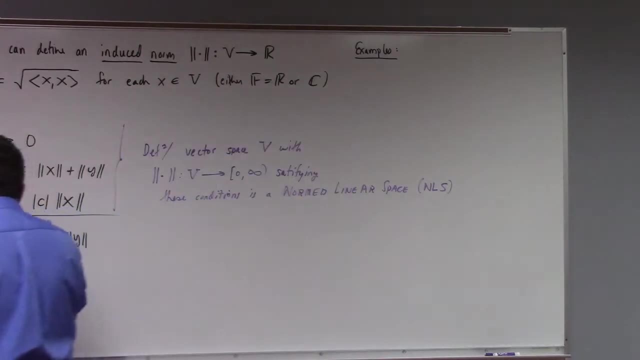 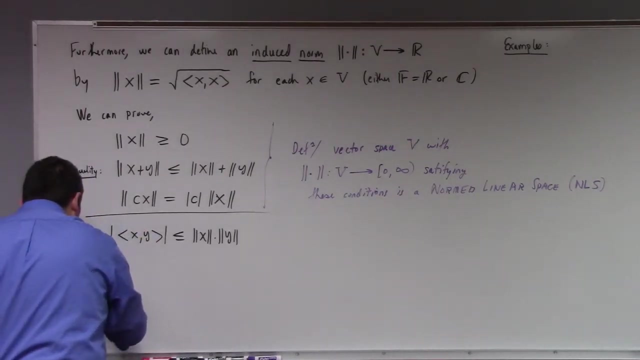 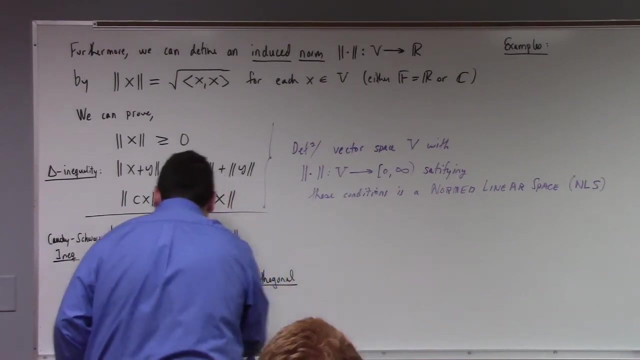 So let's do that. It might also be fun to throw out one more definition that we can study as we go on here. Vectors x and y in an inner product space v are orthogonal if the inner product of x and y is zero. 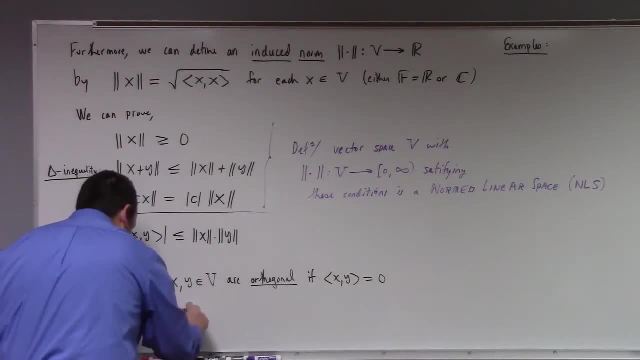 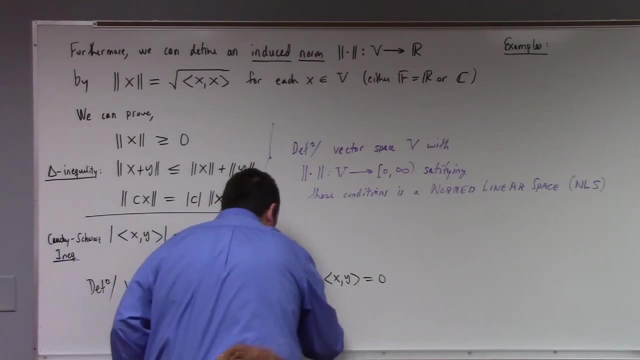 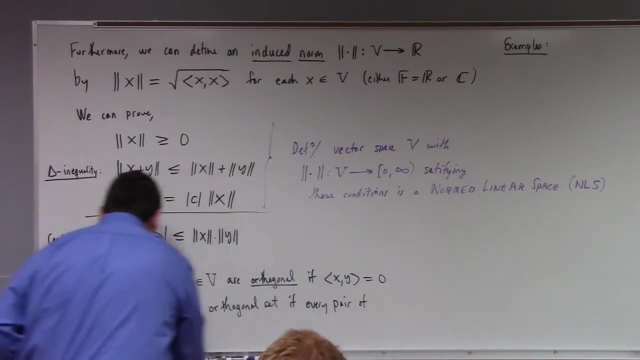 S, a subset of v, is an orthogonal set if every pair of vectors in S are orthogonal. So you take any two vectors in S, take their inner product, you get zero. That makes the set orthogonal. So let's look at some examples. 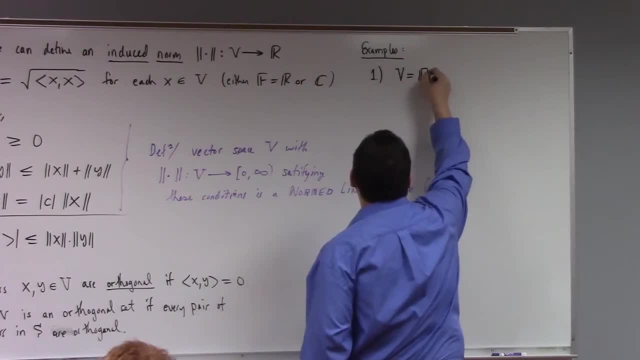 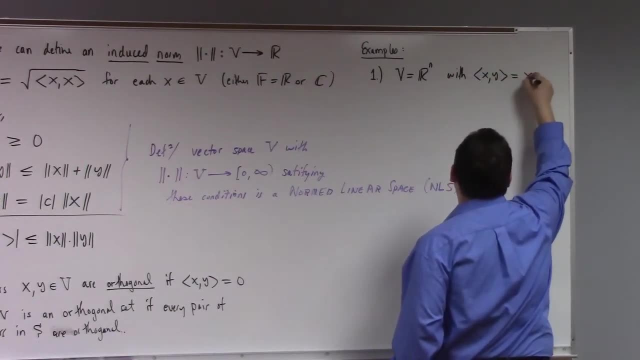 Example number one would be v equal to Rn, with the inner product of x and y just being x dot y. So just the plain old dot product is an inner product. In fact, that's really what got this all started Right. Calculus 3, we studied dot product. 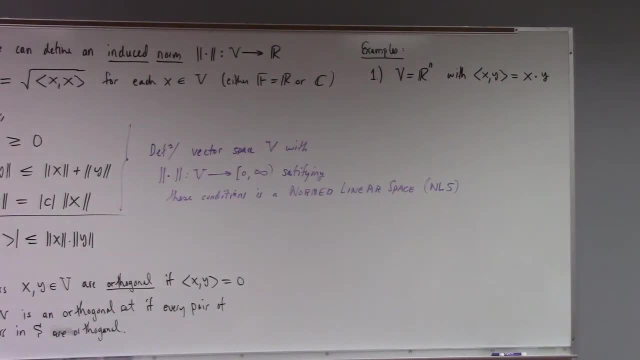 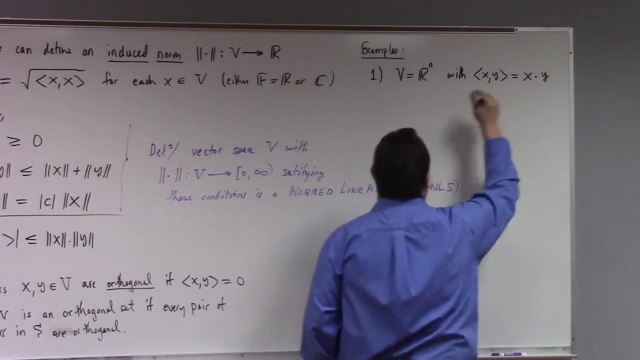 We discussed length and angle, everything in terms of the dot product. So one of our main orders of business here is to try to abstract that idea to an arbitrary vector space. But this is at the start of everything, right? So I mean I can give you a more specific formula, right? 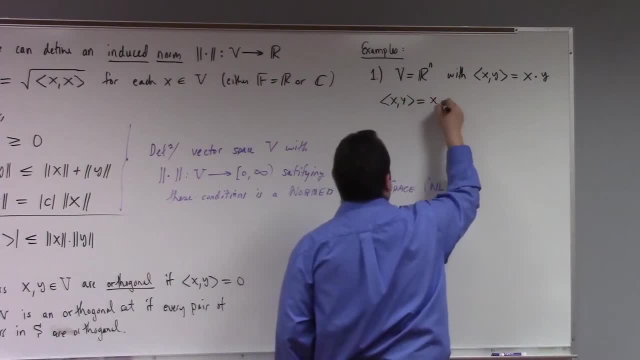 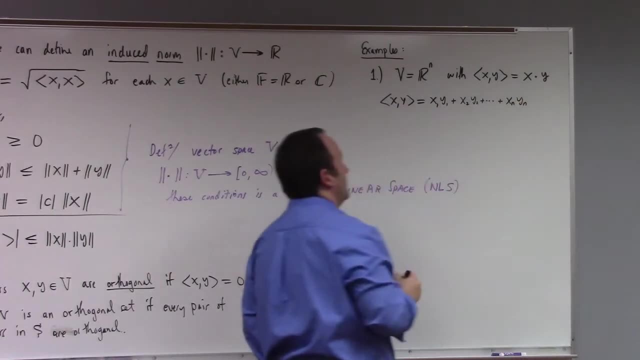 So what's x? y actually equal to? It's like x1, y1, x2, y2, plus xn, yn, right, And you can easily check that that satisfies the axioms for an inner product, right? It's commutative, which is to say that 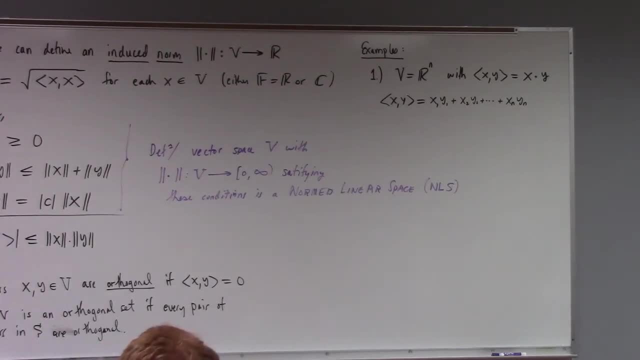 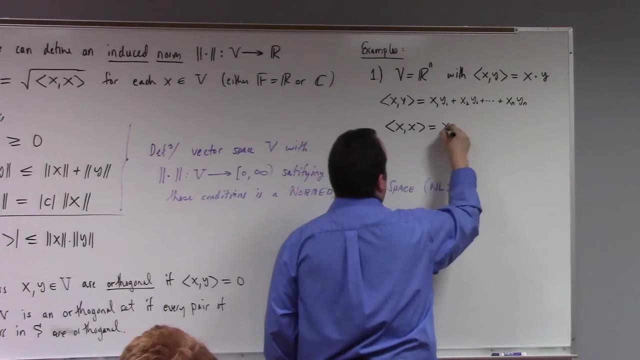 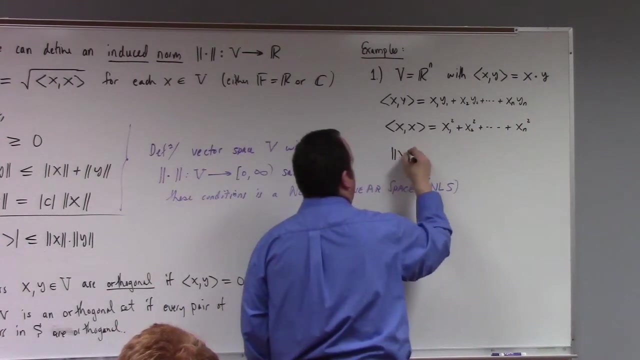 it's symmetric. And how about the inner product of x and x? What's that? We got x1 squared plus x2 squared plus xn squared right, And so the length of x is the square root of x1 squared plus x2 squared plus. 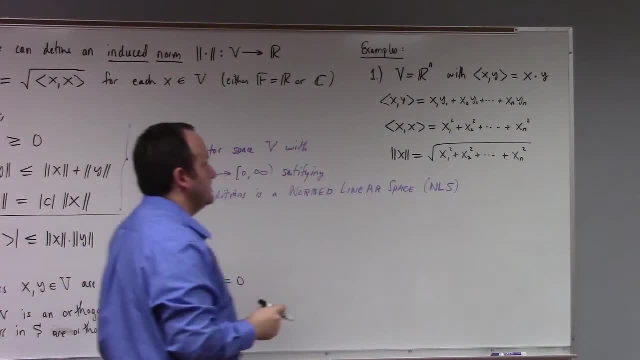 plus xn squared right. This should be familiar right? That's the distance of the point x from the origin in our n. If we look at, n equals to 2, it's just the square root of x squared plus y squared right, Or x1 squared. 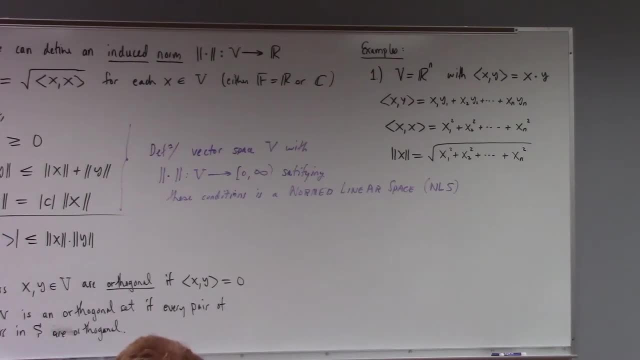 plus x2 squared, that's the distance from the origin. Three dimension: we take the sum of the x, y, z components squared, add them together. take the square root, That's the distance from the origin to x, y, z. 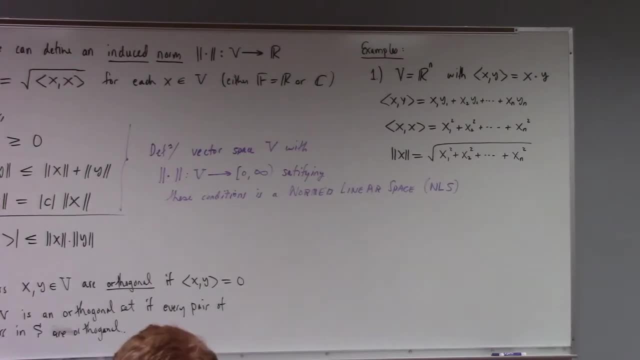 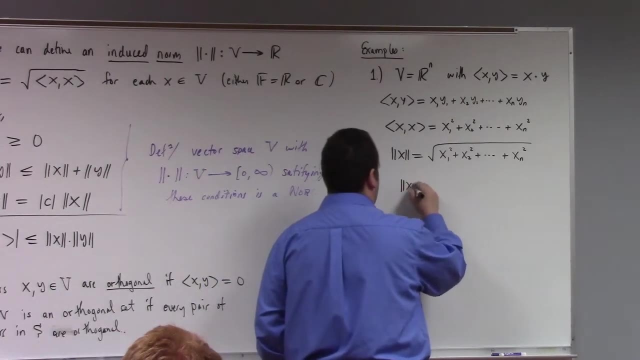 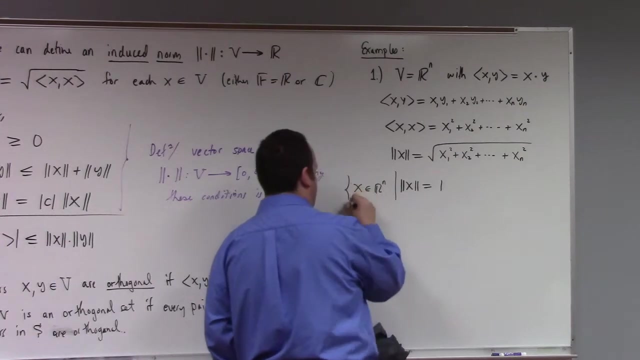 This is true right, Search your hearts, You'll find it to be true. What happens if I put the norm of x equals to 1 and say, like all x in our n, such that this, What's this? This is called. 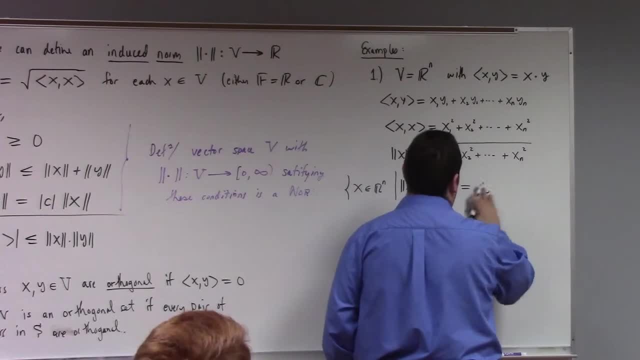 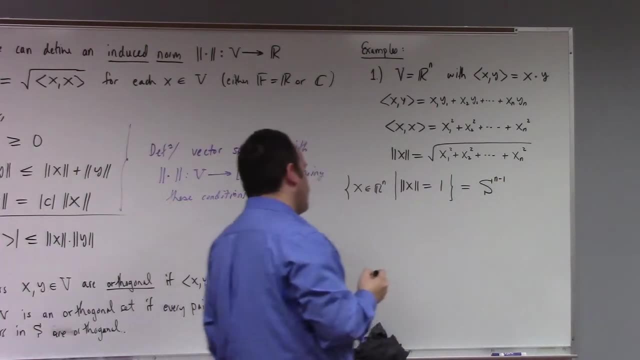 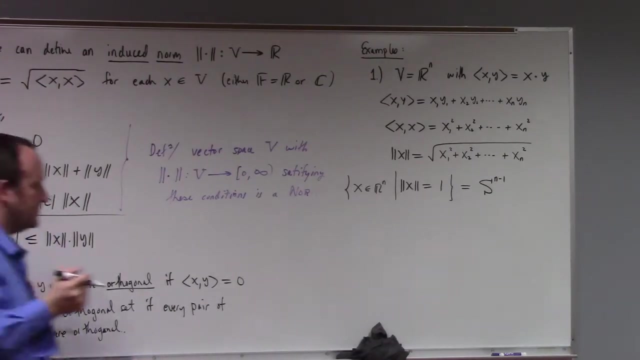 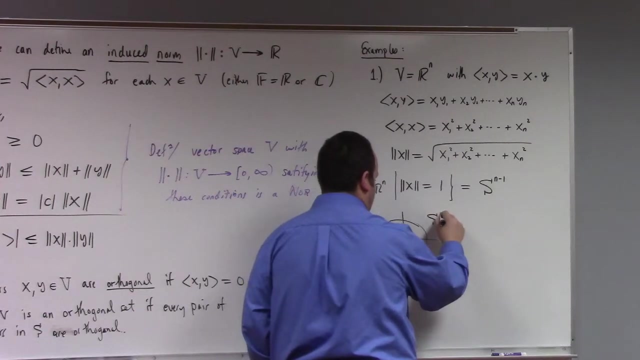 the ball. This is not the ball, This is the sphere, The n minus 1 sphere, actually. Let me explain this. So in R2, right, We have S1 as a subset. of R2 is the usual language, It's the unit circle. 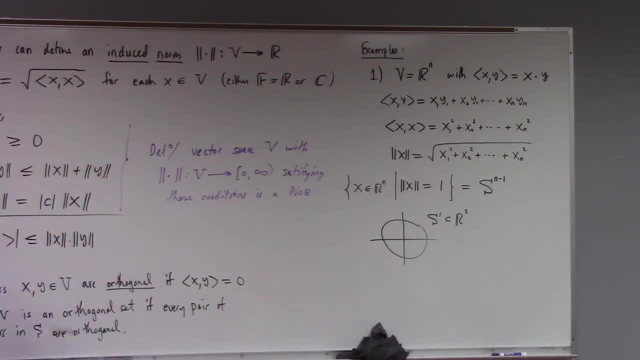 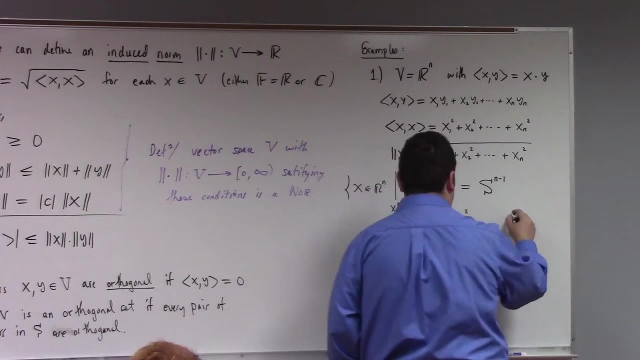 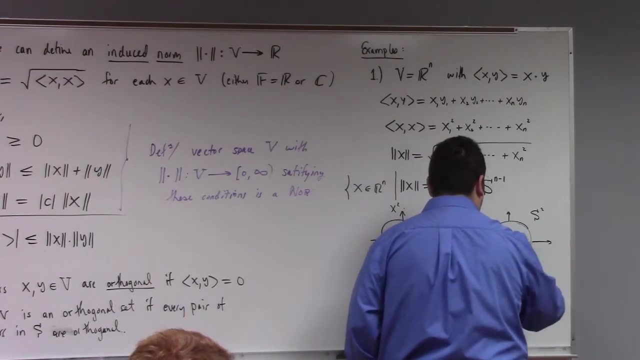 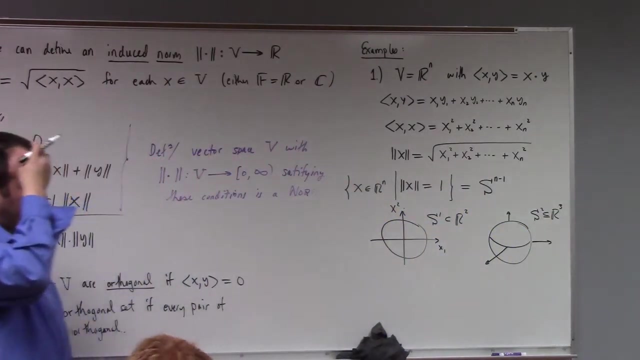 would be S1.. Right, And then How about? we can talk about S2, right Subset of R3.. We look at the collection of points that are distance 1 from the origin. This is the 2 sphere, But we could just as well define the. 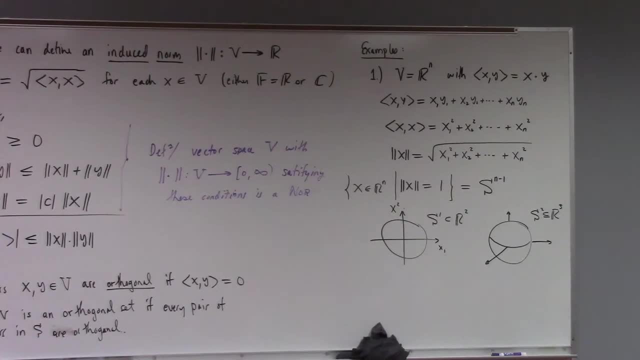 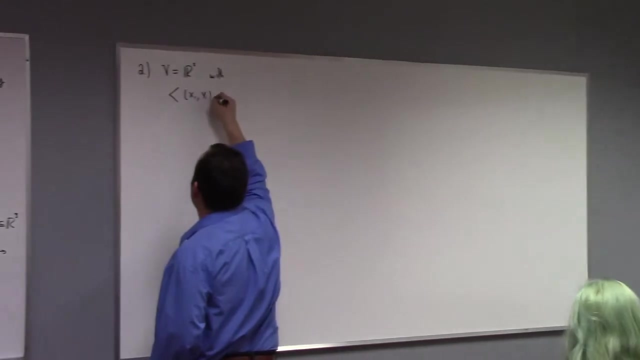 n minus 1 sphere. in Rn, Example 2, We get to take v equal to R2, let's say, for the sake of discussion, with the inner product of, let's say, x1, y1 comma, x2, y2 to be the sum. 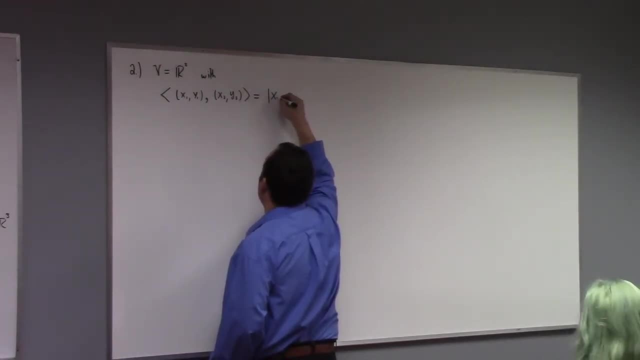 of x2 minus x1, things like that. Oh, i'm an idiot, that's not what I want. Sorry guys Stink. Oh, i'm sorry guys, i'm getting off track here: x1, x2 plus 2 y1, y2. 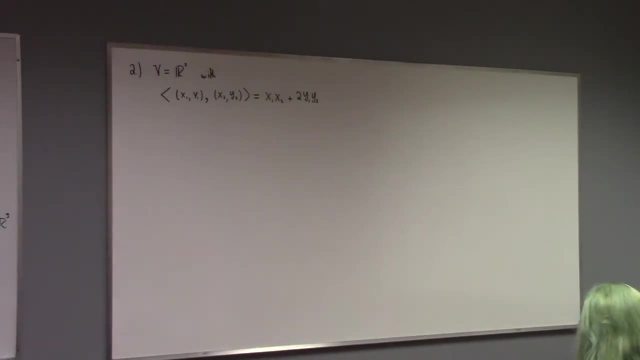 I mean, here's a different example. this is not the dot product right, it's something else. I put a two right, but if you sort through the details here, you can prove that and I'm you'll forgive me if I erase that. let me just let me like try to be consistent with my notation so you can. 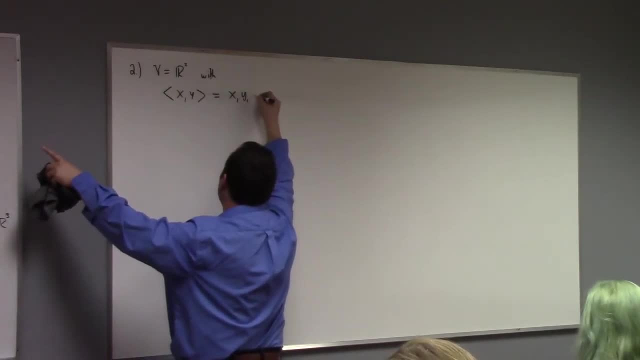 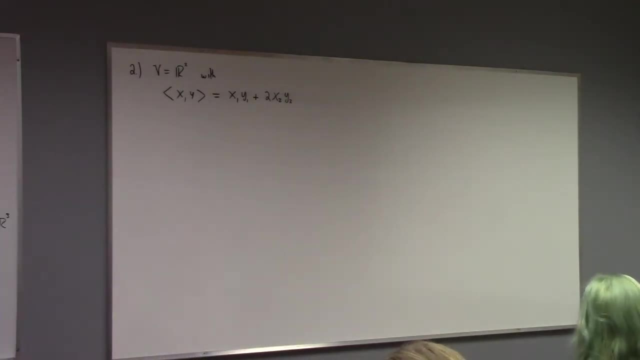 make the direct analogy more complete: x1, y1 plus 2, x2, y2, sticking with my nomenclature from example one. all right, so if this is a rather different inner product, right? I mean, is it an inner product? what happens if you take X with? 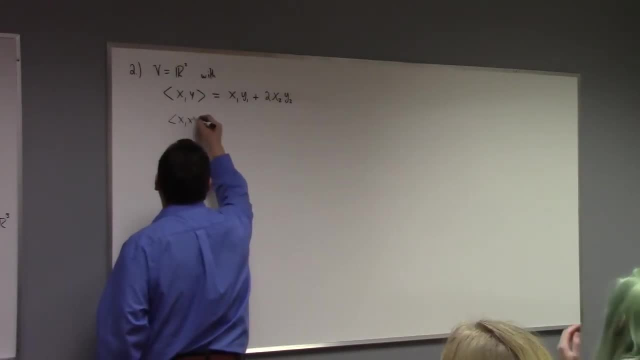 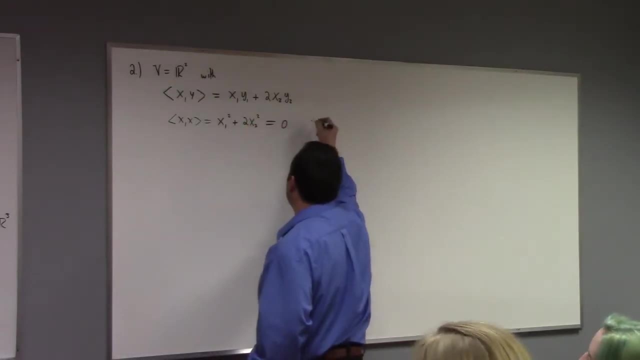 X. what do you get right? if you set this equal to 0? that's going to be 0 if, and only if, what? yeah, x1 equals to x2 equals to 0, right? so I didn't state it that way, but this is something that has to be true for an inner product is that it's only 0 if you. 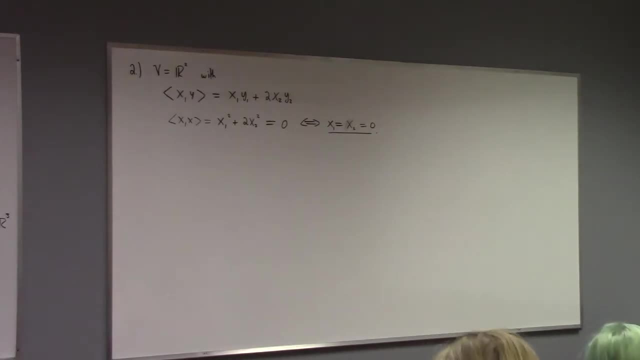 the inner product of X with X is only 0. if you put X equal to 0- that's a theorem that I have in the notes and you can easily see it's symmetric right, so there's symmetry. you can check linearity, right? so this is an inner product. what's? 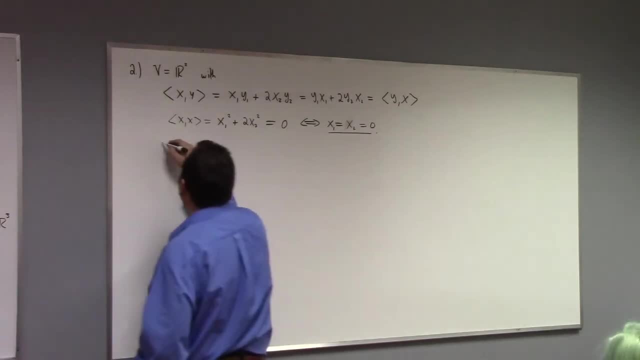 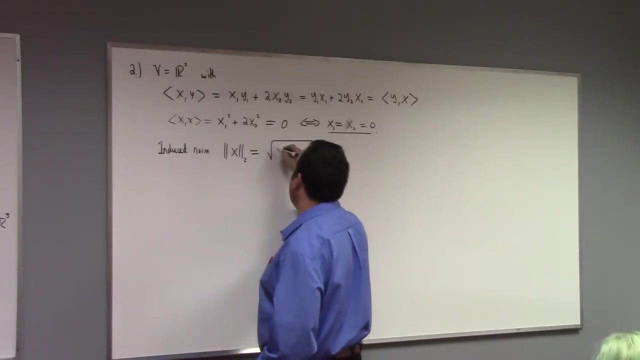 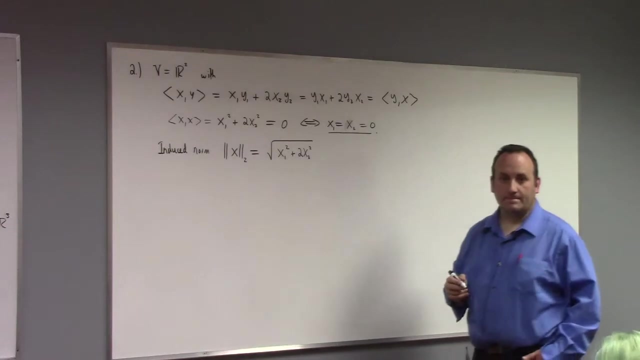 the induced norm here. well, if F, France, x1 and Y 2- cervix and Y 1- are going to get too long, or then if we look at the length of X, let's say sub 2, for example, to okay, that would be the square root of 1. 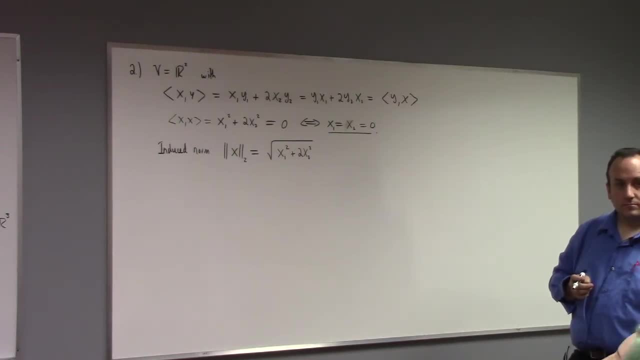 X x 1 squared plus 2x squared right. yep, yeah, You need to prove it for all four conditions. Yes, all four conditions. I was saying you can check the linearity. I have not done everything Fair enough, yeah. 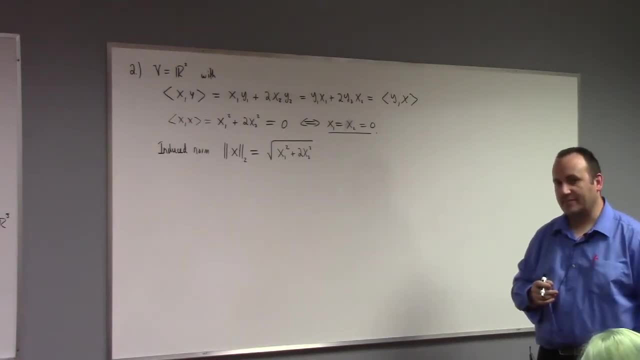 I just checked a sample condition. It's not a complete proof. no, OK, great. So this would be the norm induced for this inner product. What would the analog of a circle look like with respect to this notion of vector length? What's a circle? 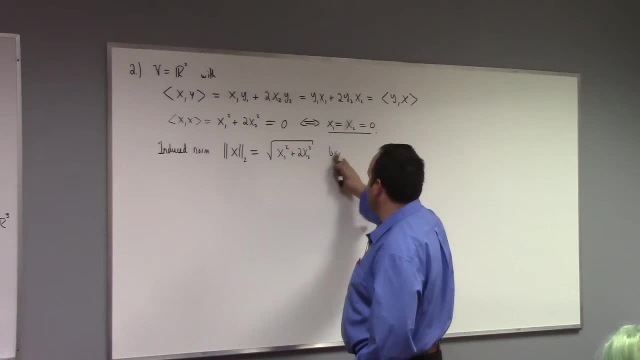 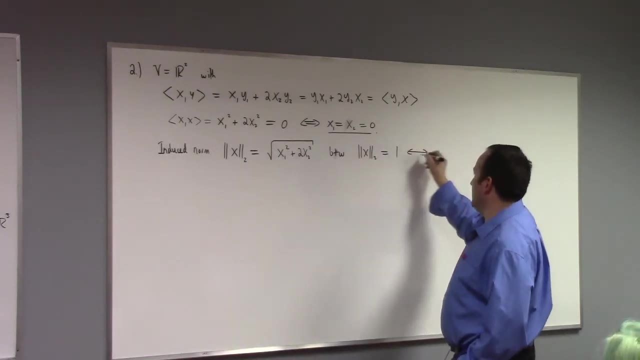 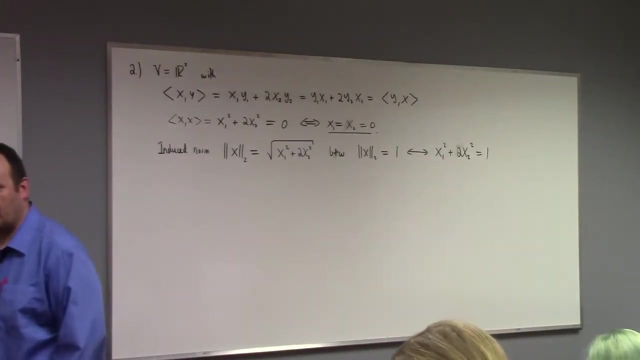 See, if I set this equal to this norm, equal to 1, that means that x1 squared plus 2x2 squared equals to 1.. So, with respect to this notion of length in the plane ellipses- And that's what the norm of the plane ellipses- 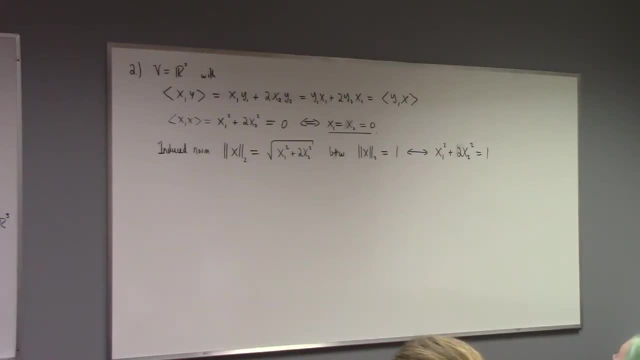 play the role circles do. So you have the question is: what defines a circle? Well, if the circle is a set of points that are the same vector, the same length from the origin, as defined by your norm, then a circle might look different in different choices of geometry. 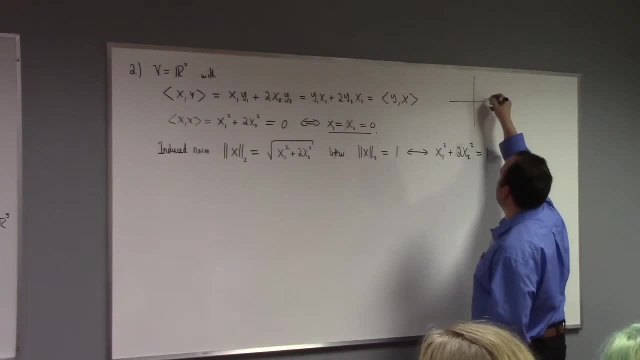 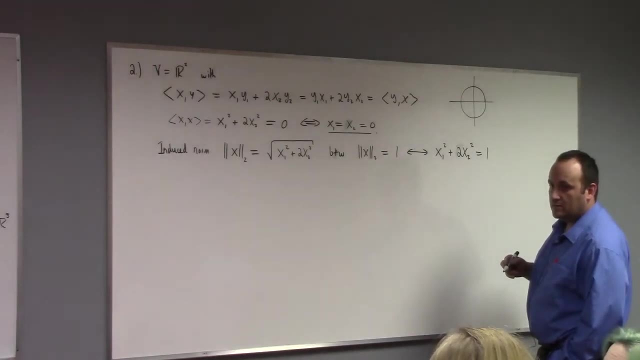 You can define different norms on the plane. So this is the. You know, It's like this, right, Yeah, OK, So say that not every norm has an inducing inner product, but does every inner product induce a norm? Every inner product induces a norm. 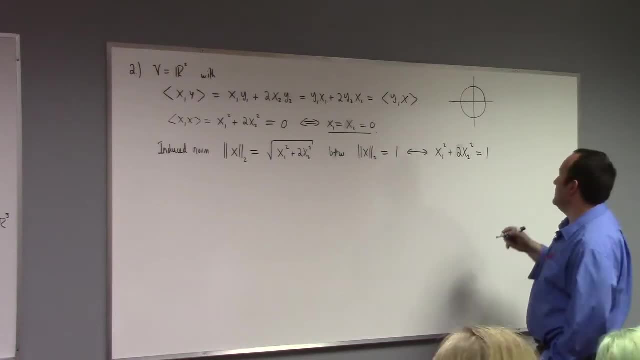 However, not every norm is induced from an inner product. That is true. In particular, I can define the length of x to be the value of x1 plus the value of x2.. This is the so-called one norm, The sum of the absolute values of the components. this, in fact. 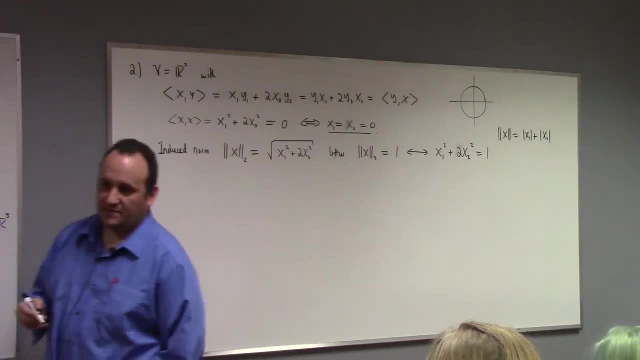 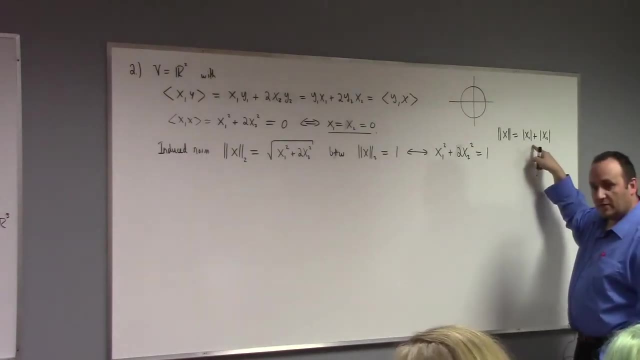 would not be induced from an inner product. It's not obvious, but it's not obvious that that's true, But it is in fact true. But what's interesting is, if you use this notion of inner product, the circle with respect to that one norm is a diamond. 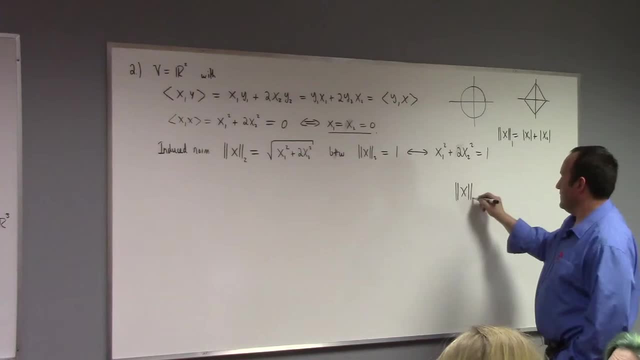 If instead you let the length of a vector, the so-called three norm would be the cube root of x1 cubed plus x2 cubed. This is the so-called three norm If you look at the quote unquote circle with respect. 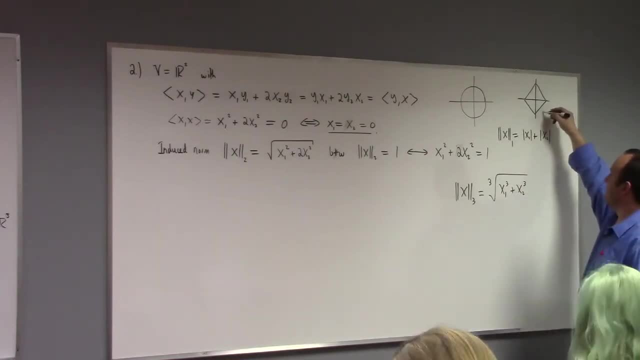 to the three norm. so this is essentially: p equals to 1.. This is the Euclidean p equals to 2.. This is p equals to 3. The circle with respect to the p equals 3 norm. well, I have to draw all of them on the same thing. 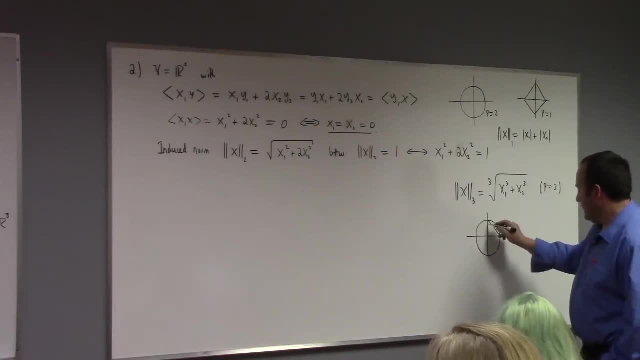 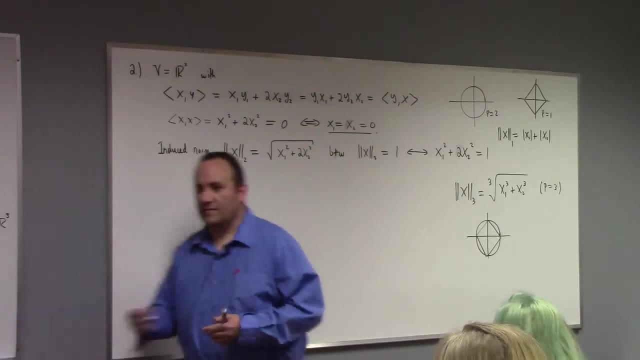 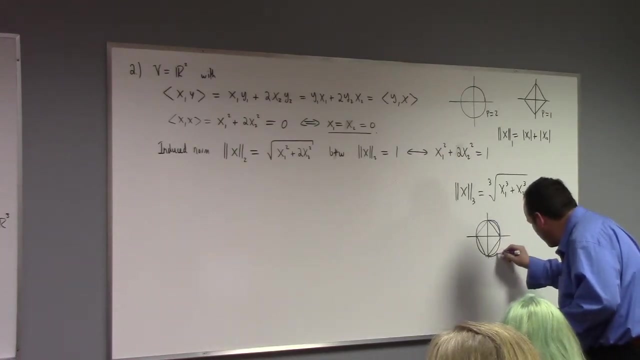 So here's the circle. Here's the one norm. The three, the circle with respect to the three norm is the one norm. Here's the one norm. Here's the one norm. Looks like this: It's like a circle that's been blown out a little bit. 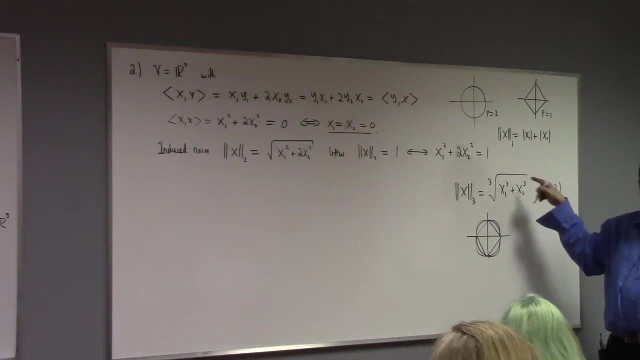 If you were to replace 3 with 4, take the fourth root of the sums, of the fourth powers of the components. that also defines a norm, so-called four norm. If you take the limit as p goes to infinity, you get something called the sup norm or sup. 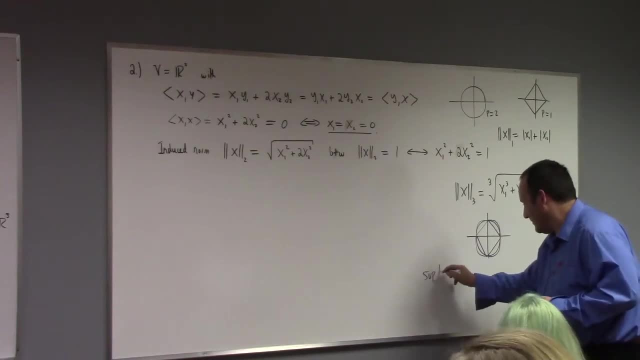 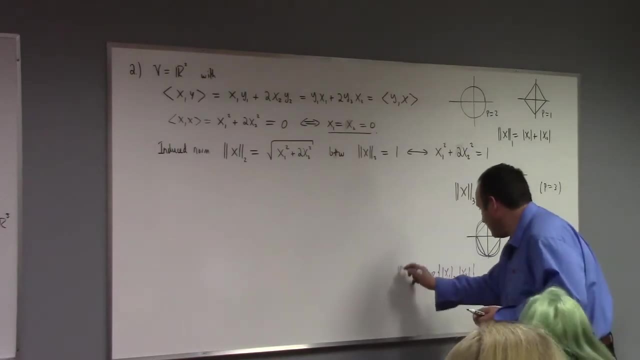 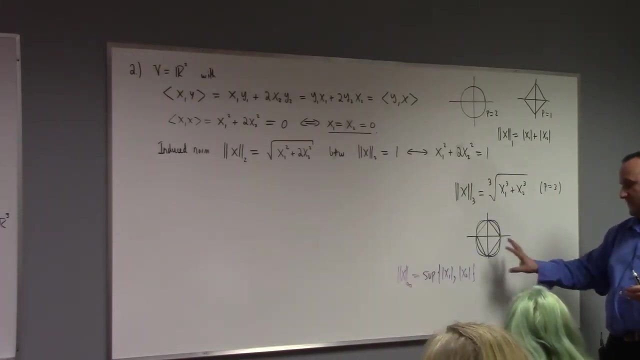 So you take the supremum of x1 and x2, or the max, if you like, since that would be the same. This is the p equals infinity norm And the circle. there is a square, In other words the set of vectors in the plane, which. 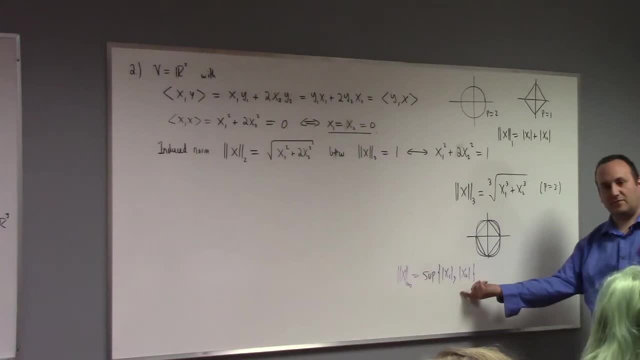 have. distance 1 from the origin, as measured by this notion of norm, is actually a square. so you know we're entertaining the idea that distance can be differently defined than the Euclidean distance. at the same time, my title for the chapter is Euclidean geometry, so I'm mostly focused on that. 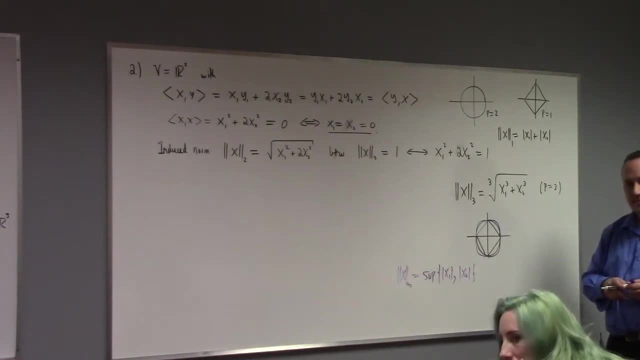 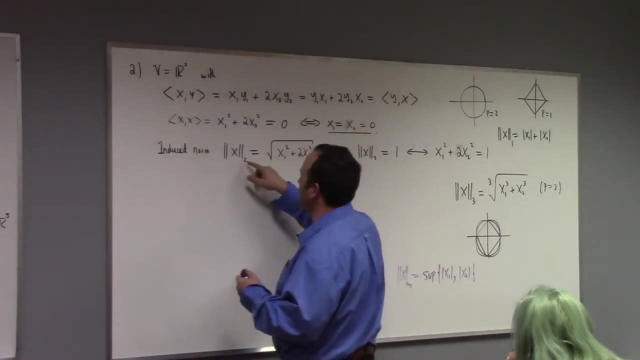 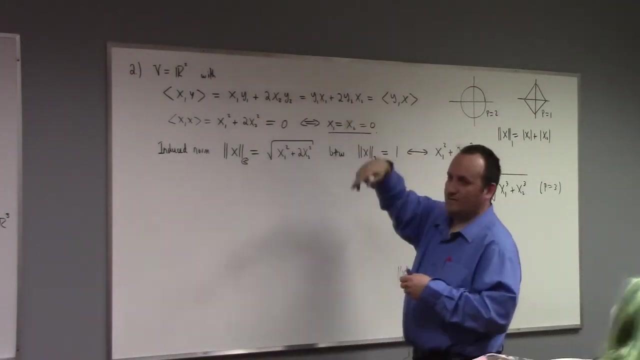 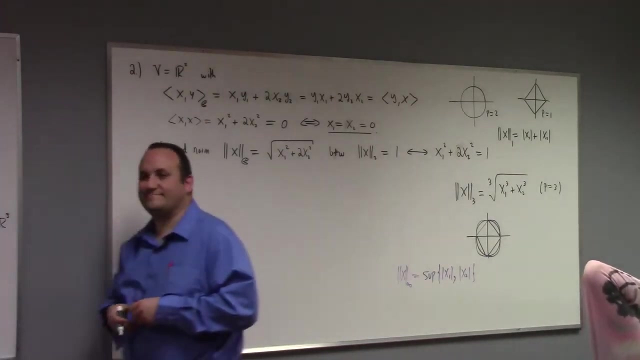 yeah, oh, this was. this was a different sub to this. I should call it sub pac-man, because this is a weirdo. I mean, we put a pac-man here. this is a different inner product, obviously, than this one for different exam. yeah, yeah, no, there's no. 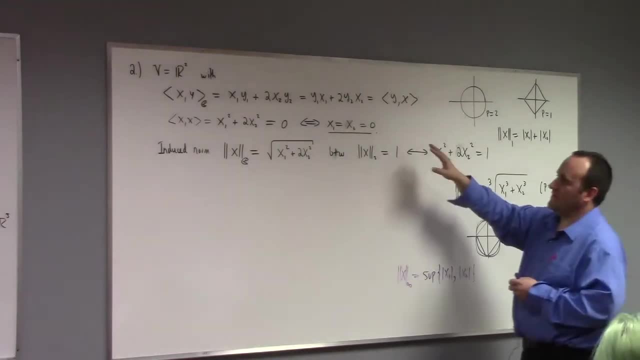 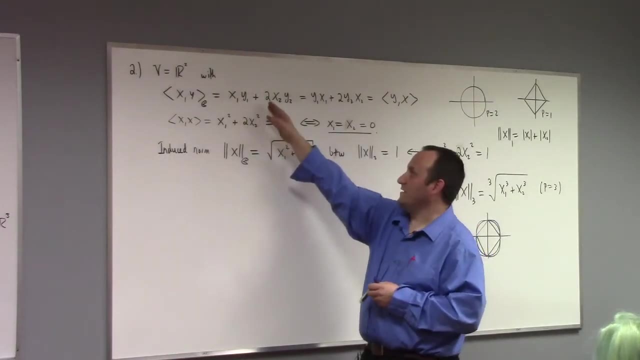 reserved notation for this. I mean this. this could be something like the inner product, could be something like a score in a class. maybe you've got an assignment which has weight one. the first assignment has weight one, the second assignment has, like weight two. you might look at this sort of inner product for such an 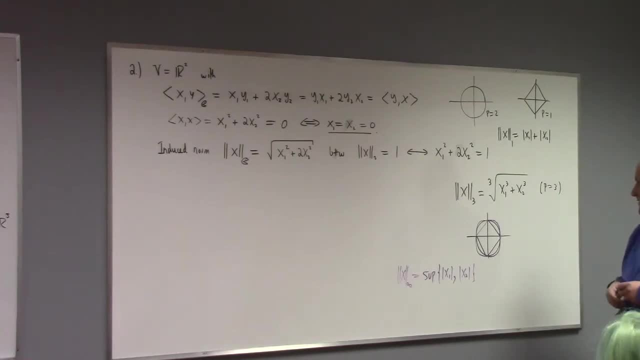 application as that, but I'm fond of this discussion and I'm wasting entirely too much class time on it. you'll apologize, but I find it very amusing that as P goes to infinity, you get a square. see, I guess that's also sort of a fair run, because if you've ever taken a 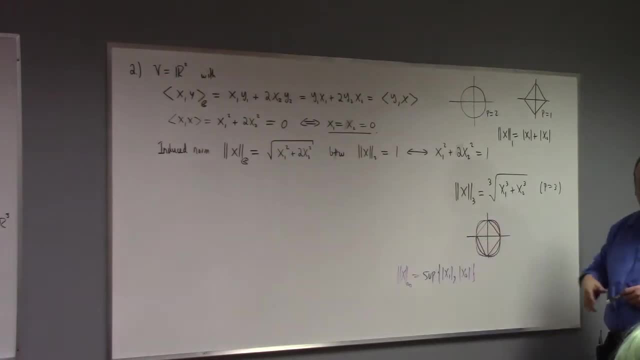 philosophy class you'll hear philosophers throw this phrase around. it's like squaring the circle. it's an absurdity. it's not an absurdity, you just use the soup norm. we've been doing it for like a hundred fifty years of math. where you guys been, it's not a big deal. the square is a circle with the right. 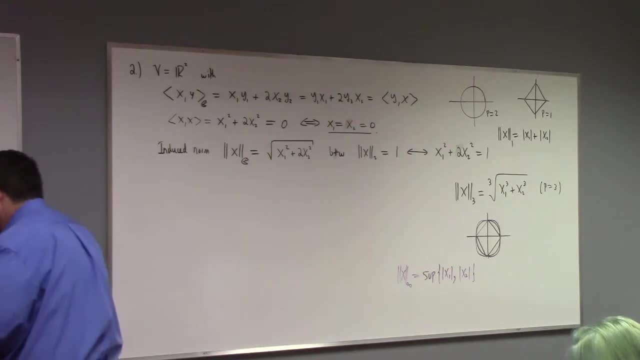 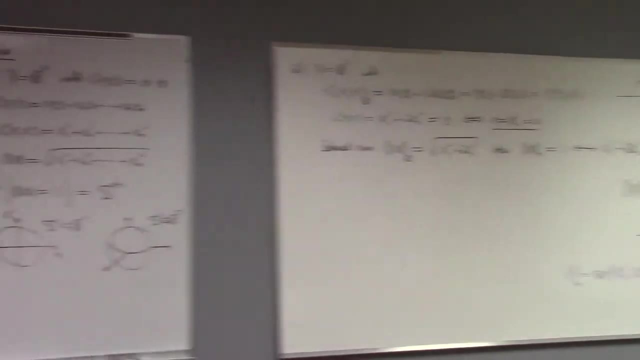 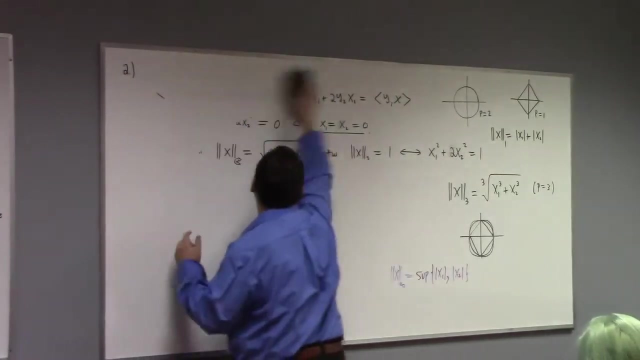 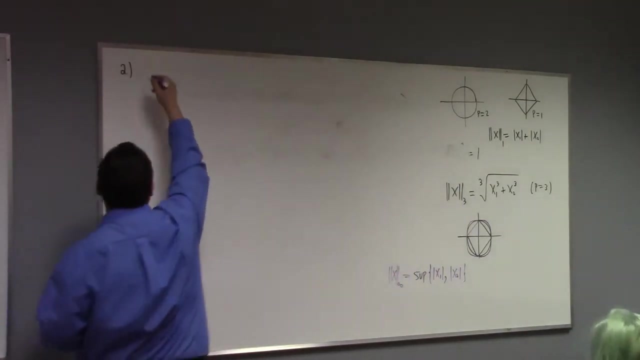 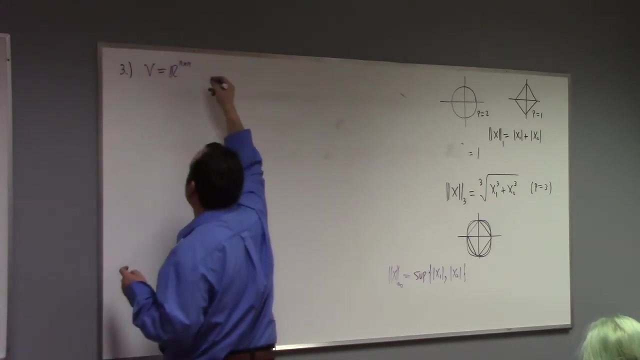 understanding of what a circle is generally. but yeah, they won't care. but um, So let me move on with my examples. All right, So V equals to Rn by n. So here you might want to define what's the inner product of A and B. 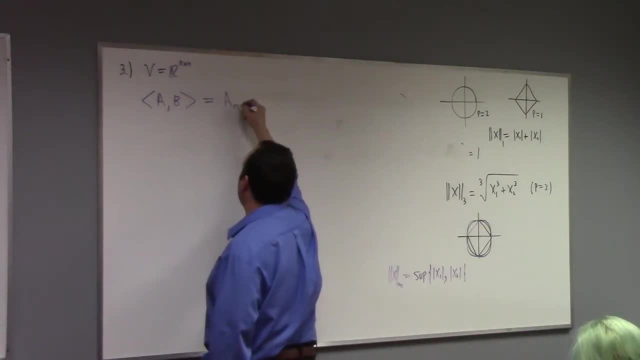 Two square matrices. Guess what you do? You do A11B11 plus A12B12 plus da-da-da-da-da plus ANNBNN. In other words, just take the n by n matrix, string them out as like they're a big old vector. 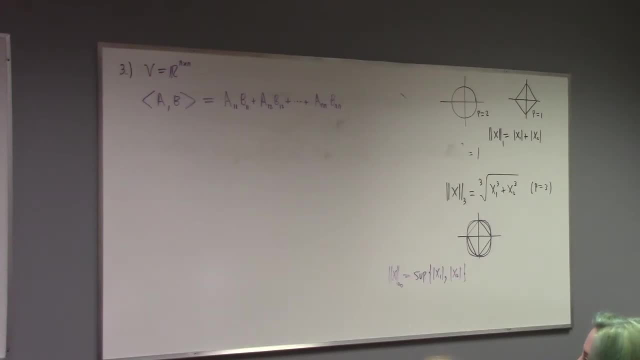 and take the dot product of those vectors. Now that's great, But it turns out there's a super sneaky formula for this And it's just this: It's the trace Of AB transpose. That actually is the same formula. 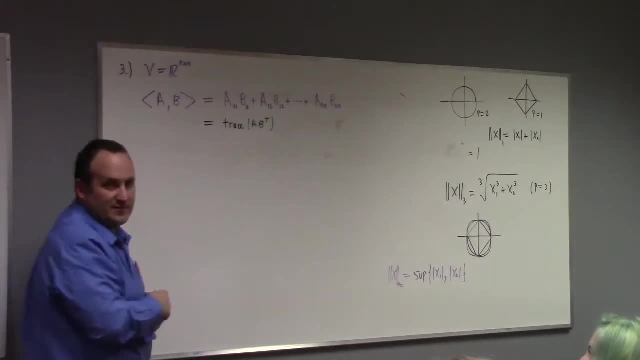 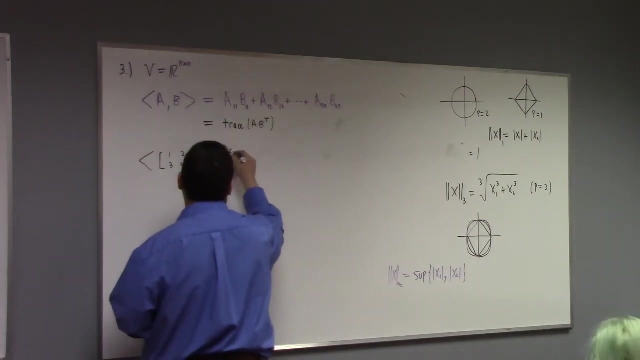 If you don't believe me, would you believe me? Oh, an actual example. Okay, so Let's see here: One, two, three, four- My favorite matrix- Eight, six, seven And then X. Here's the question. 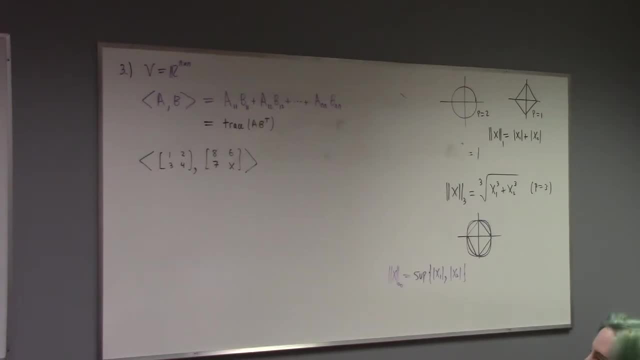 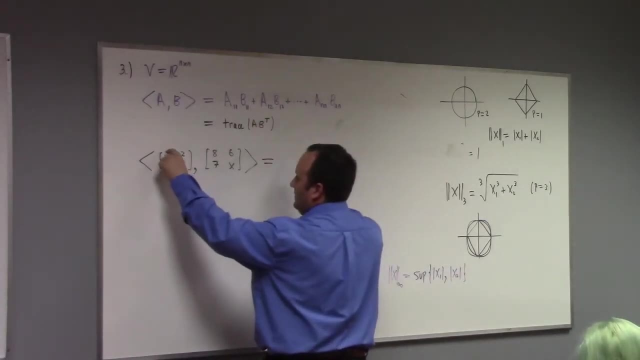 Choose X, if possible, to make these orthogonal. Can we choose X to make these matrices orthogonal? All right, so here's the definition. This is eight plus 12 plus 21 plus 4X. Do you see what I'm doing? 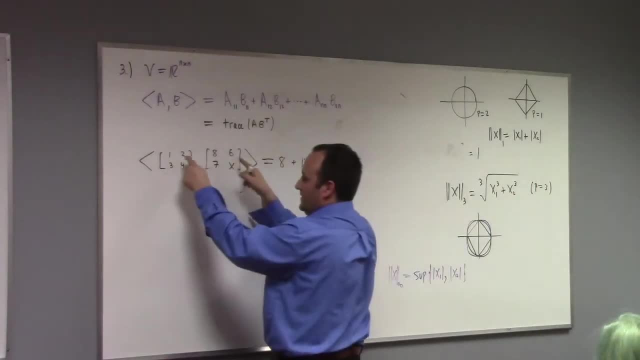 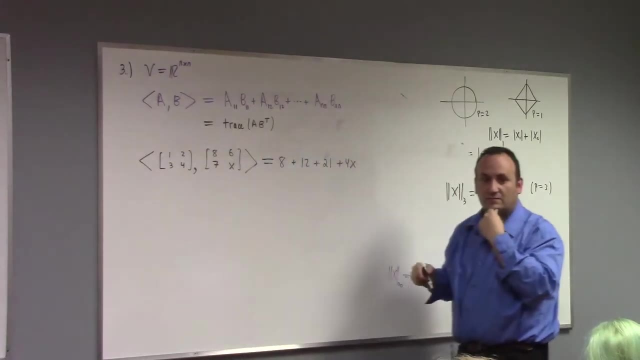 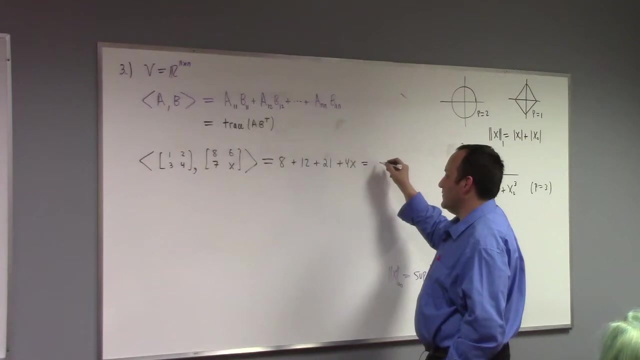 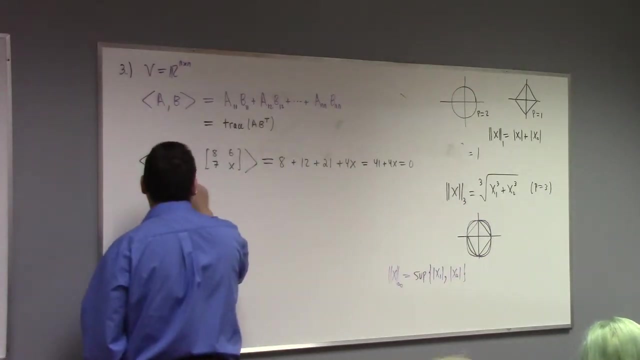 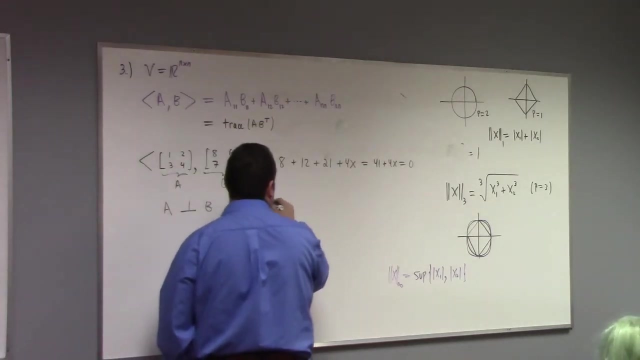 I'm just I multiply corresponding, so I don't actually use this formula to do it, I just do it directly from my initial definition. so if I, what do? I got 2041. so if this is, if this is a and this is B, to make a perpendicular to B, we choose X, equals. 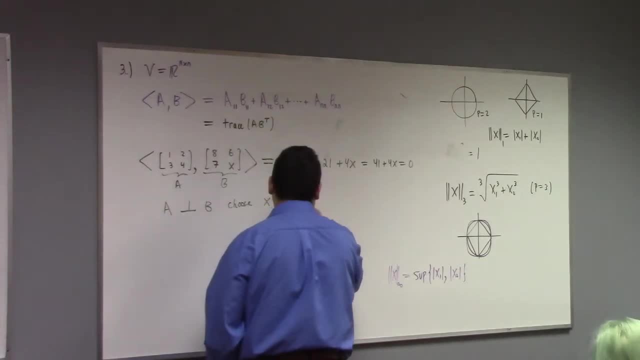 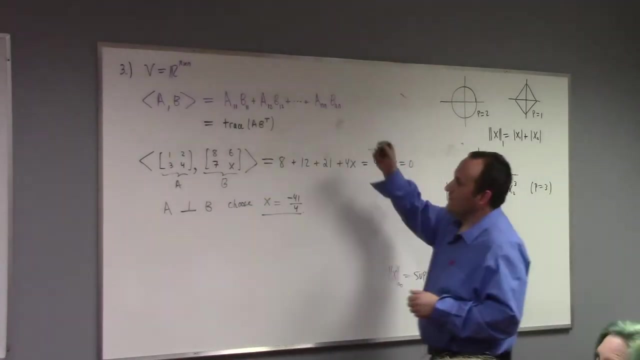 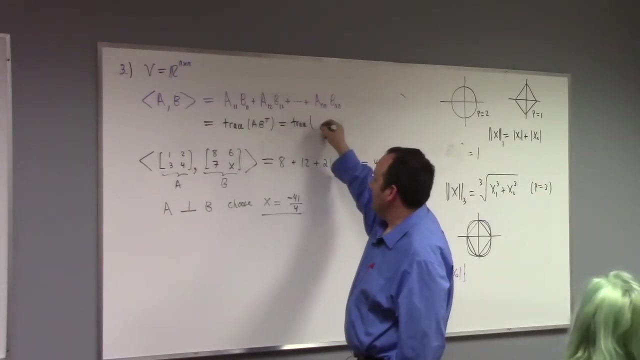 2 minus 41 over 4 make that a test question. I do tend to ask things that are at this level of computationally on the next test, does it is something that happens. look, how would you prove symmetry here? so this is what. this is the trace of what a B transpose. 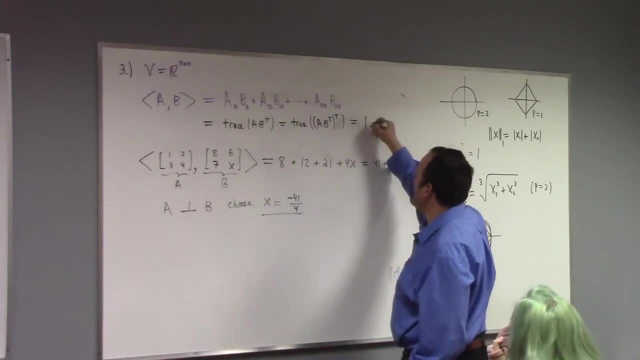 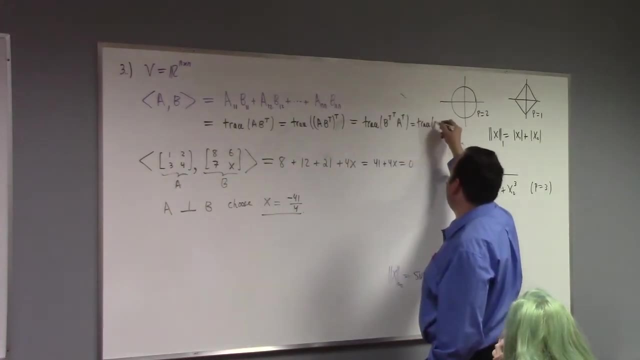 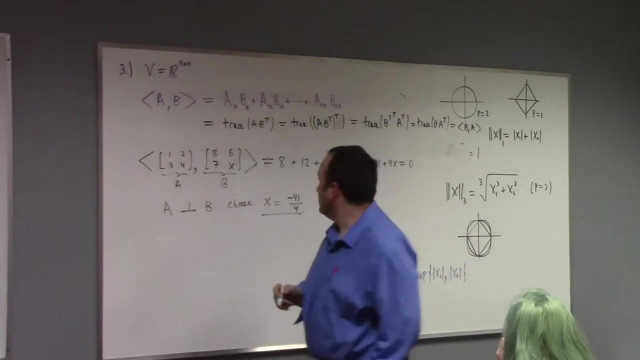 transpose right. is a matrix equal to its transpose? no, not generally speaking. but what is the trace? trace is the sum of the diagonals. the diagonal is fixed under transposition. this calculation is reasonable. so there's why it's Emmett, why it's symmetric. what's the length of a 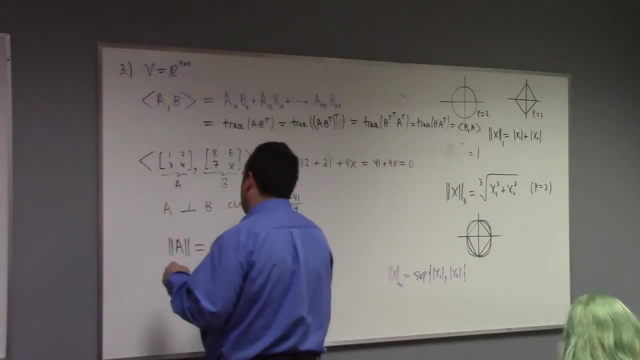 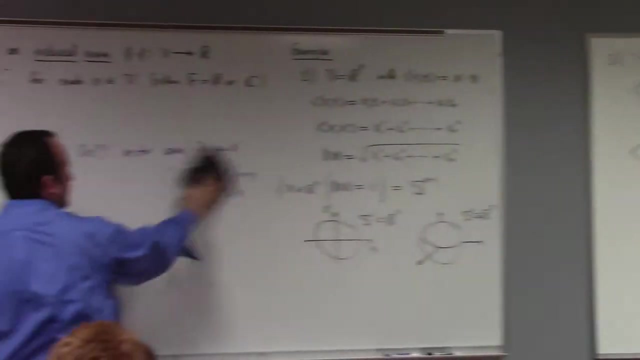 that's the length of a here. this is the so-called. by the way that this has a name, it's called the Frobenius norm. all right, you, you, you, you. so my next example, we. so this is: you know, did you do, do, get grief, poor life choices here. 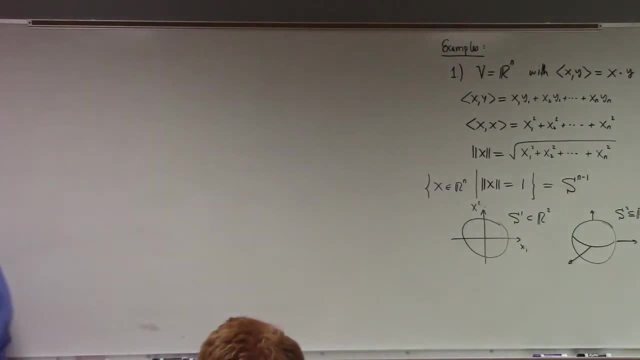 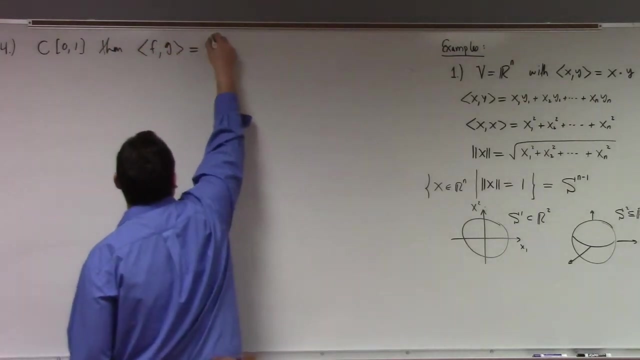 you, you, you, you. if we look at continuous functions from 0 to 1, continuous functions of 0- 1, then you can let the inner product of f and G be equal to the integral from 0 to 1 of f, of X, G, of X, DX. 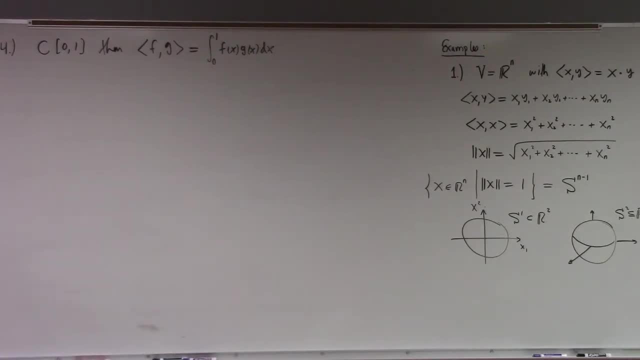 you thanks, thank you. this is an infinite dimensional example because the continuous functions through 0 to 1 are not a finite-dimensional vector space, right? But nevertheless, this is a definition you can give and it's easy to check that you know. 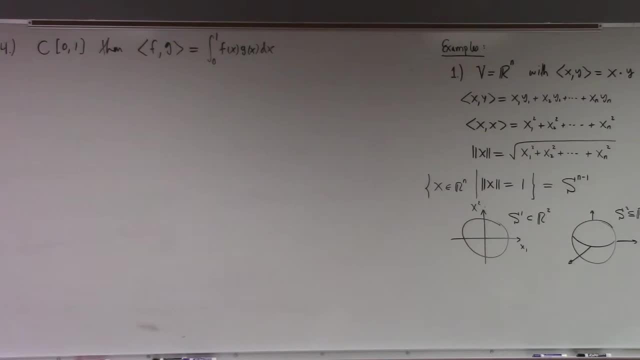 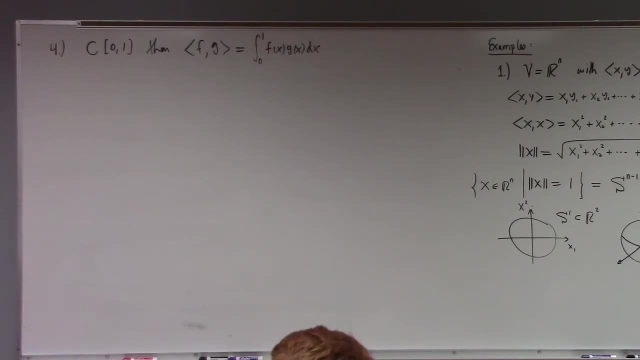 first of all, C0, 1 is a vector space, right, because the sum of continuous functions is a continuous function. The scalar multiple of continuous functions is continuous, right? So you can check that. that is indeed a vector space And it's easy to check the axioms here, right? 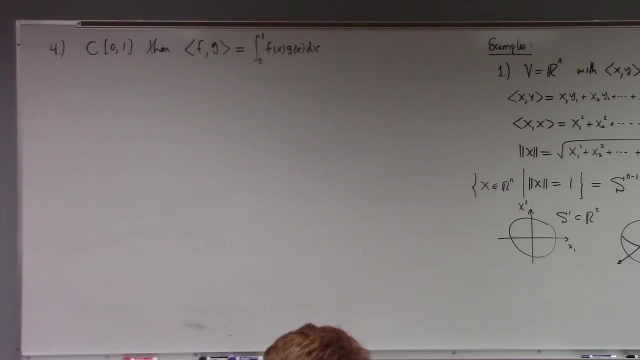 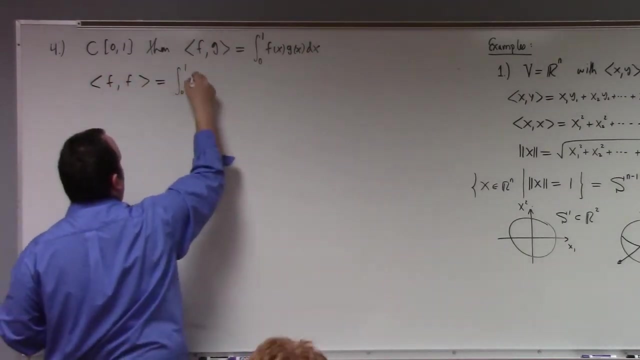 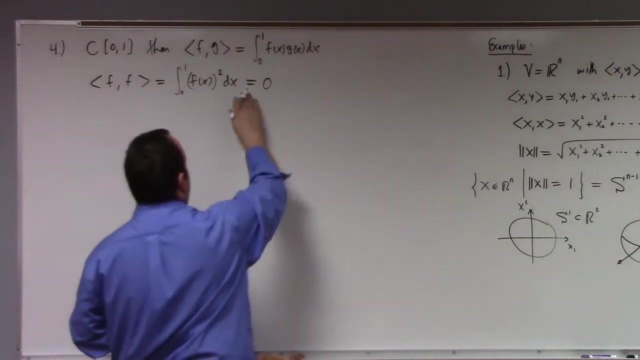 Like additivity, just corresponds to that corresponding property for integration. right, And you can pull constants out of an integral. Why is it that? the one that's kind of interesting to look at is what happens when we take f with f, I mean, is it possible to have? 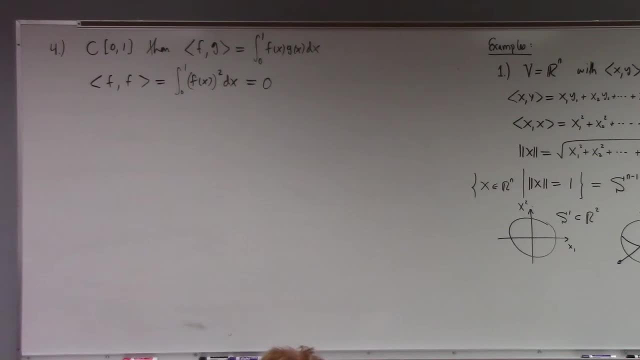 If this is equal to 0, what does that tell you? Yeah, It means f of x has to be identically 0, right, Because f is continuous. It can't just be non-zero at one point. It has to be continuous in a neighborhood of that one point. 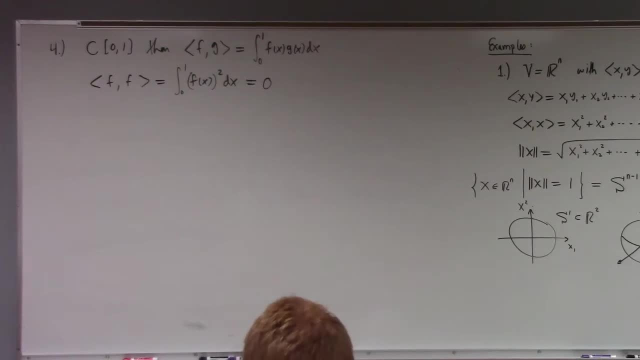 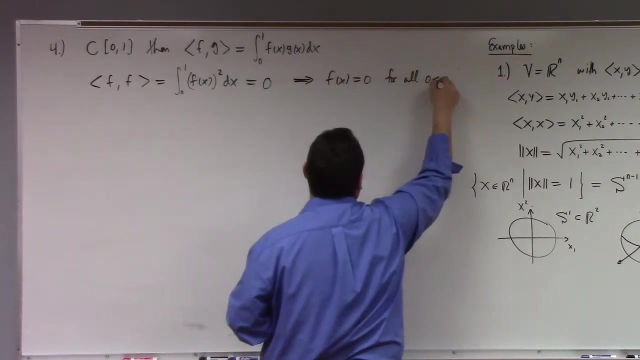 which means, when you calculate the integral, you get something non-trivial. So the only way we could have 0 here is that that implies that f of x is equal to 0 for all. All right, So you know a particular example. 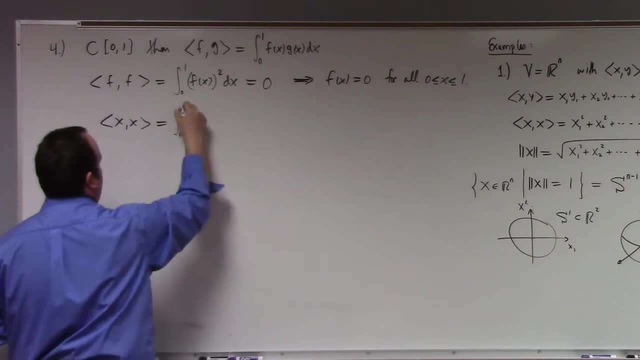 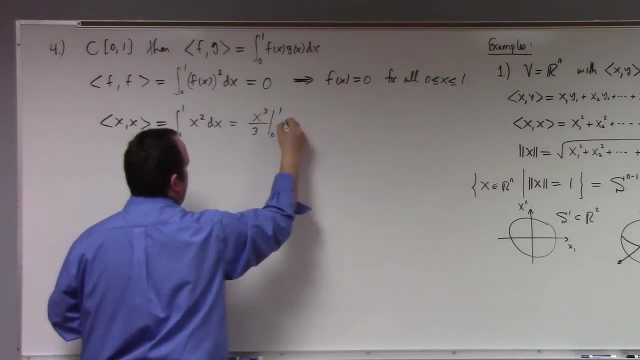 if we look at the inner product of x and x, we have the integral from 0 to 1 of x squared dx, yeah, Which is x cubed over 3, evaluated from 0 to 1.. This is the part of calculus you guys like. 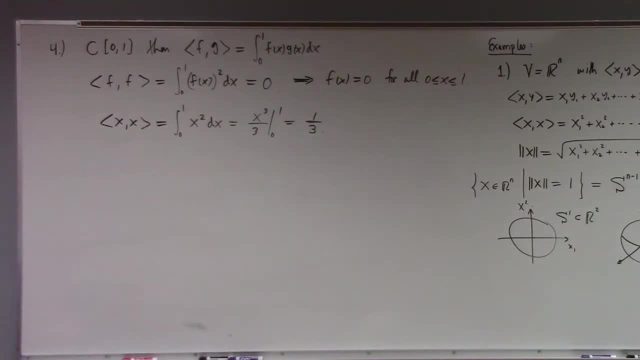 Am I right, One-third? So what's the length of x? The norm of x in this context is 1 over the square root of 3.. x is a vector of length 1 over root 3 in this context. Now my choice of 0 to 1 here is somewhat immaterial. 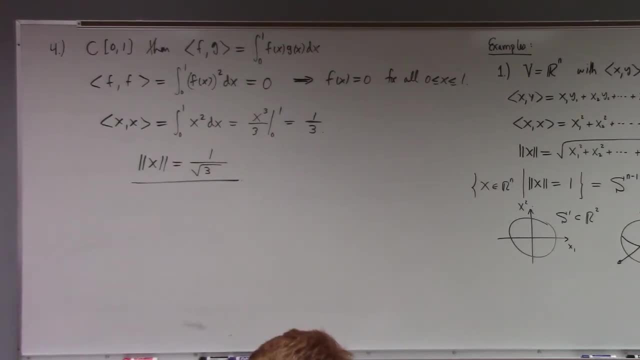 As we go on, I'll look at Things from minus 1 to 1, and it changes the calculation a bit. Instead of getting 1-third, you get 2-thirds here and so forth. but All right. next up. 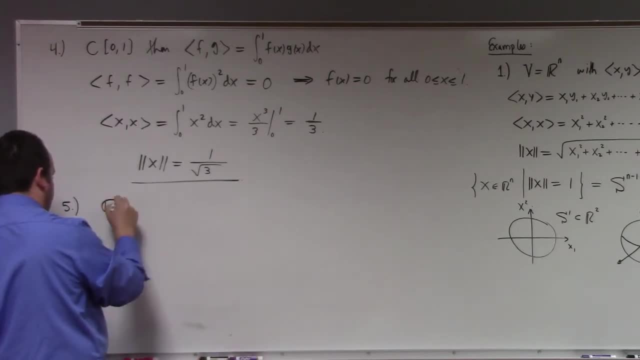 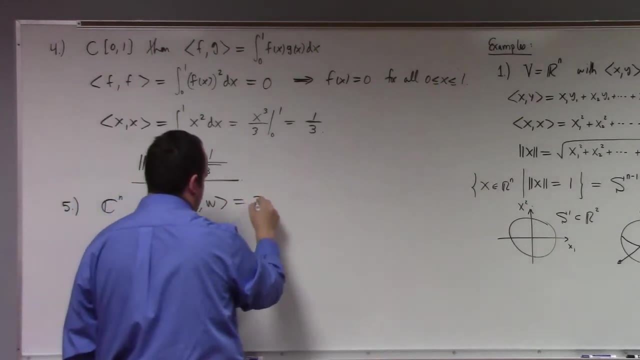 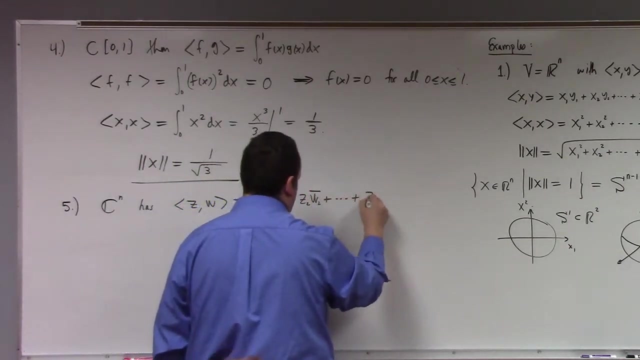 If we looked at Cn as the inner product of Z and W, equal to Z1- W1 conjugate plus Z2, W2 conjugate plus Zn- Wn. You need the complex conjugate there in order to get the necessary sesquilinearity. 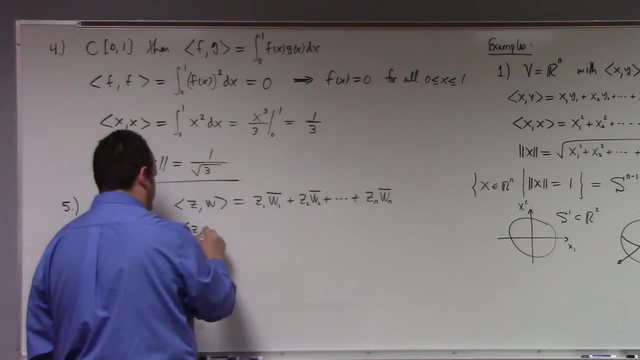 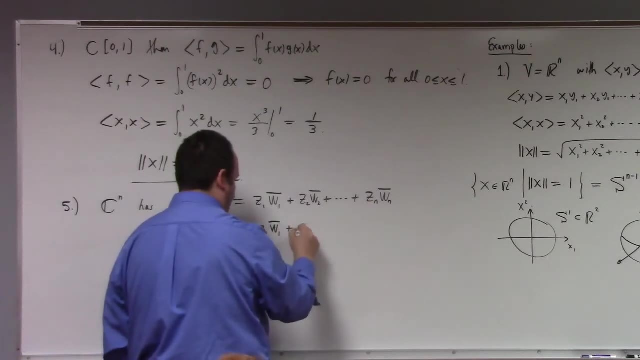 Like what happens if we take the complex conjugate of Zw. How does complex conjugate work? One of the reasons we have this course is because it's a pretty complex course. It's a pretty complex course, It's a prerequisite for 421, is to try to get you comfortable with this. 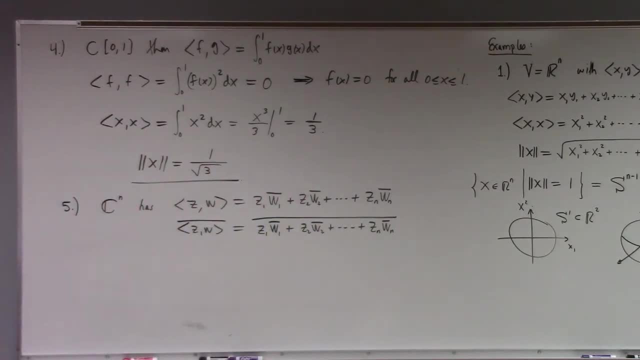 You should never comfort yourself with this idea that complex is not a prerequisite for another class, so you don't need to know complex. That's just a fallacy. We do cover complex variables in other courses other than complex. It's just complex variables is where we study complex analysis. 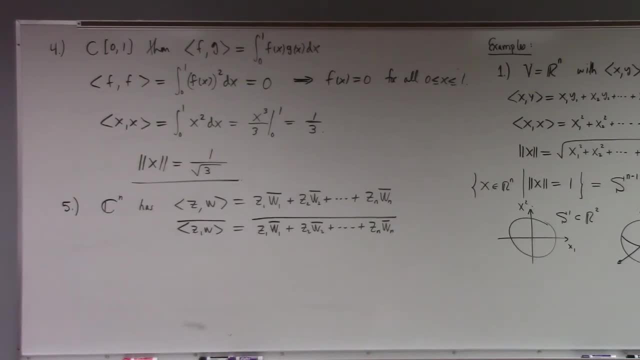 Complex algebra is in all your higher level courses, be it differential equations or this course or 421.. It's something you need to learn if you don't know already. Many of you want to be future high school teachers. This is something you need to master anyway. 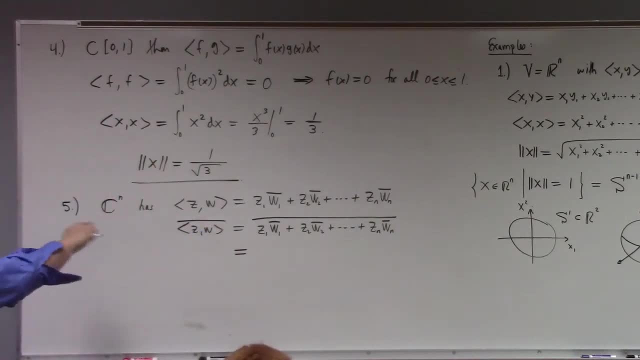 So the complex conjugate of a sum is the sum of complex conjugates. And how does that work? Remember, this is Z1 conjugate- W1.. Z1 conjugate conjugate plus Z2 conjugate- W2 conjugate conjugate. 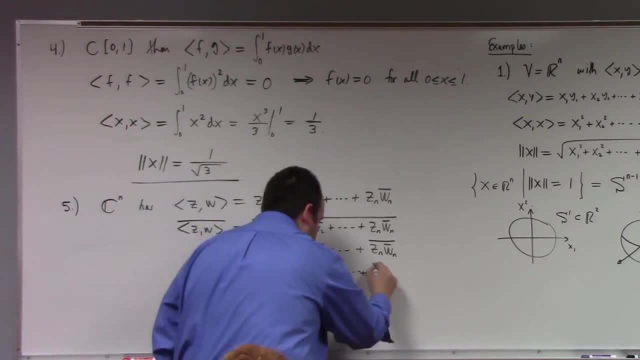 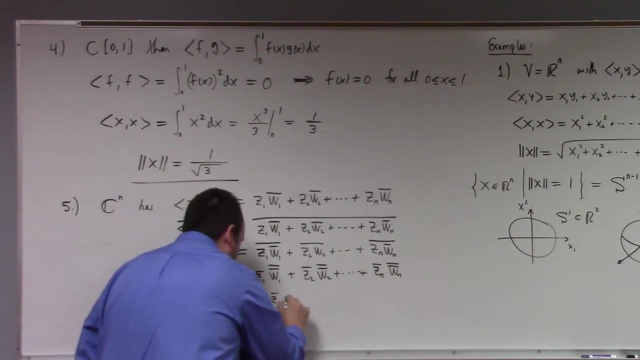 Which is kind of silly to write, because what's the conjugate of the conjugate? Just the thing again, right, So I can rewrite that. And these are complex numbers, so they commute. So what do we got After? we take the complex conjugate of the definition. properties of complex conjugate. 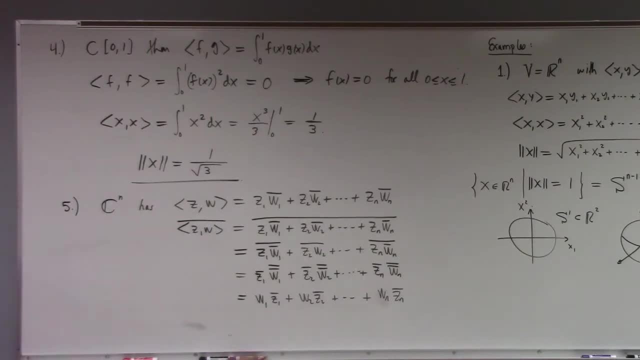 work through. what do you got? You got W is Z, Which is what we need for axiom C over here. Here I'll look at a particular one. If we let Z equals to say 1 plus i to 3 minus 4i, then what is? 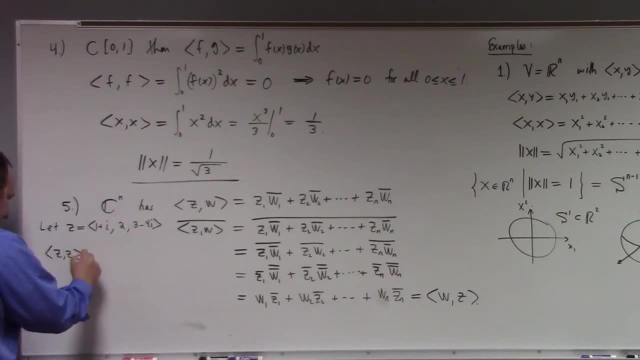 what is the inner product of Z and Z here? in this context, It's 1 plus i times 1 plus i conjugate plus 2 times 2 conjugate plus 3 minus 4i times 3 minus 4i conjugate right. 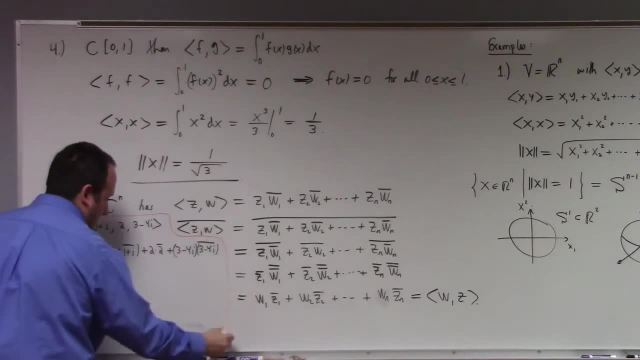 And so what's going on here? What happens when you multiply a complex number by its conjugate? What does it give you? It gives you the absolute value squared of the complex number or the modulus squared. It's the length of the complex number. squared is what it gives you. 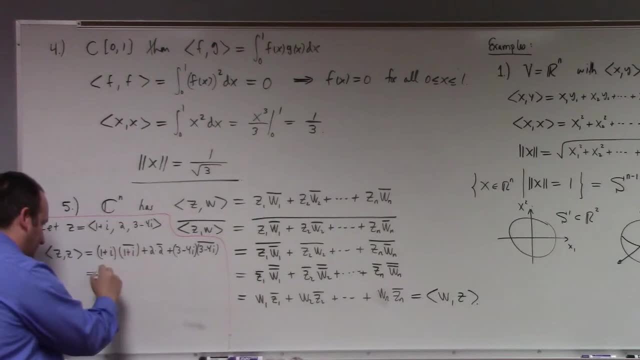 In other words, this gives us 2 plus 4 plus, well, 25.. So that's the sum. OK, So the length of the first one is square root of 2.. This is complex number with length, square root of 2.. 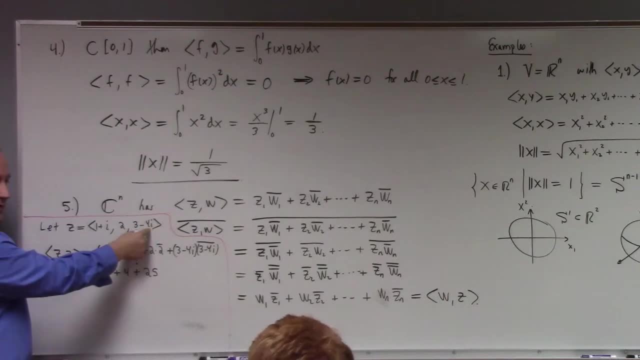 2 is a complex number with length 2.. 3 minus 4i is a complex number with length 5.. Because the square root of 9 plus 16 is the square root of 25, which is 5.. This is length 5.. 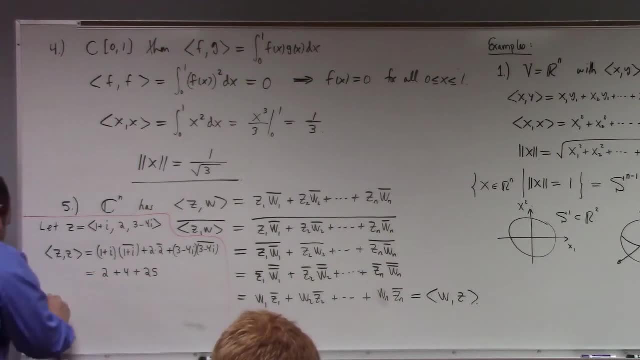 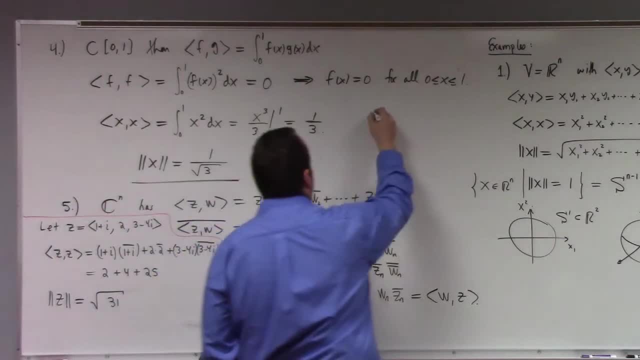 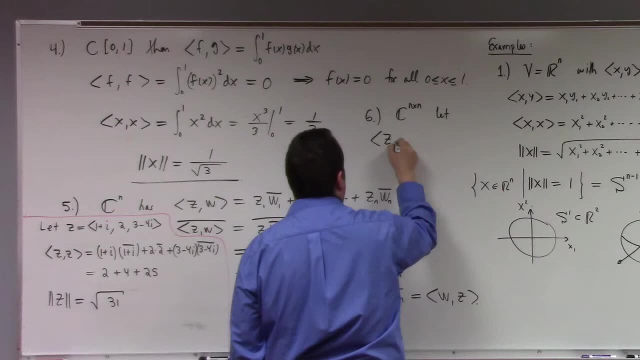 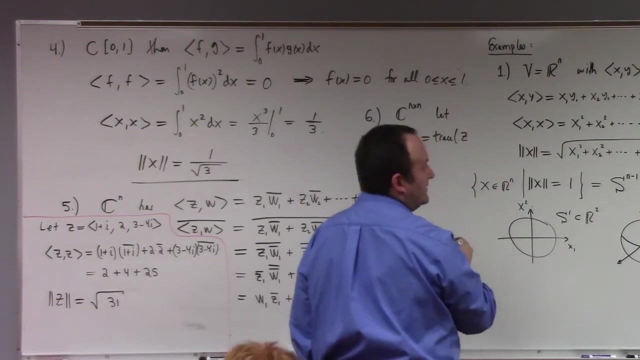 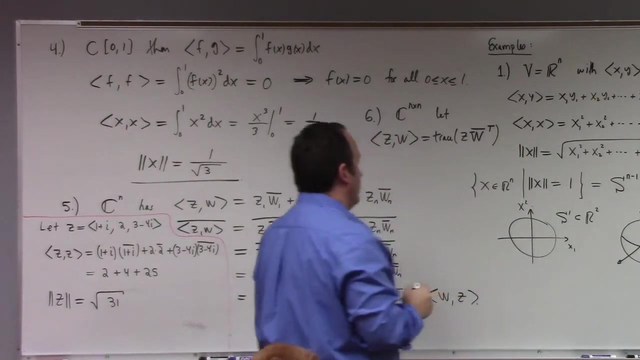 You can also 6 if you have c n by n. Let the inner product of big Z and big W be the trace of Z. How'd it go? I erased it. z w bar transpose. that is essentially just the complex inner product of the complex matrix looked at as a n squared vector. just, it's just the. 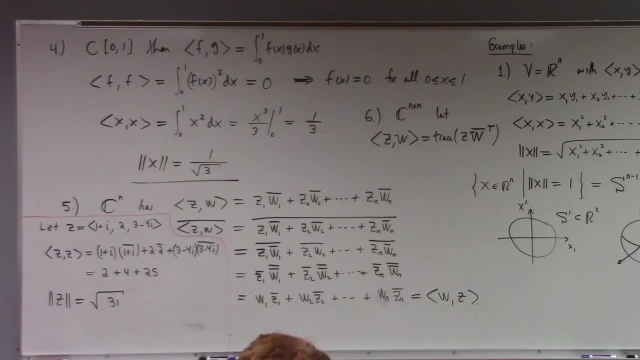 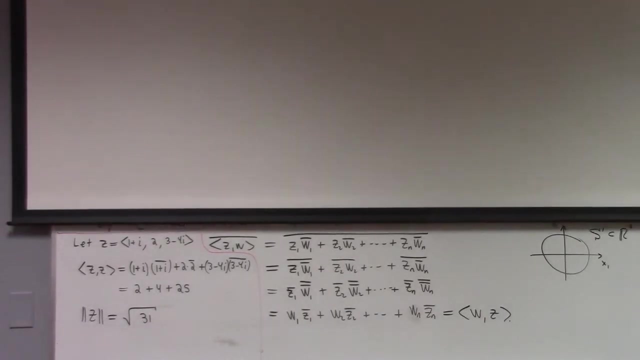 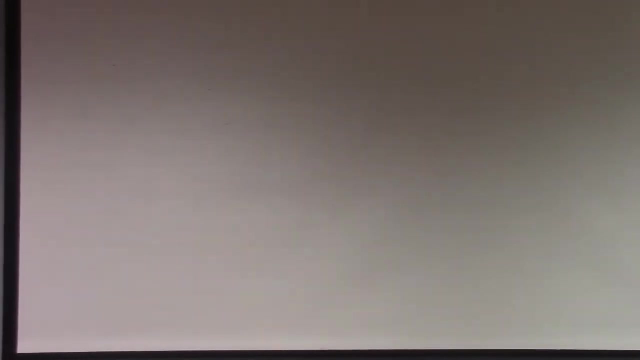 piggybacking off my previous example. oh, all right, oh sorry, should warn you. I know you're all like a lot unfulfilled at this moment because we haven't, you know, done that thing that we do yet. so let me eventually the so that you guys know. 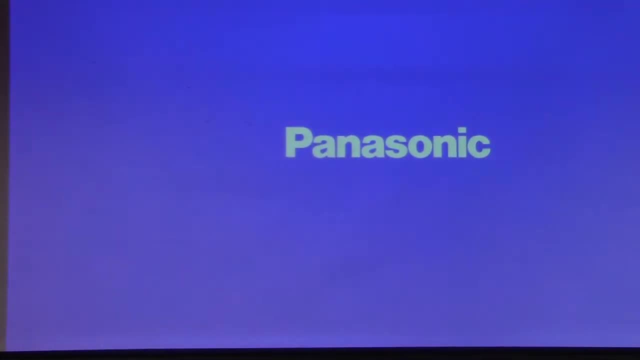 where we're, where we're going with this discussion at the moment. I'm just trying to get everything out in front of us, give you a sense of how we define inner products for our standard examples. we've pretty much done that at this point, so I'm going to spend the next 10 minutes I'm trying to recover all of the theorems. 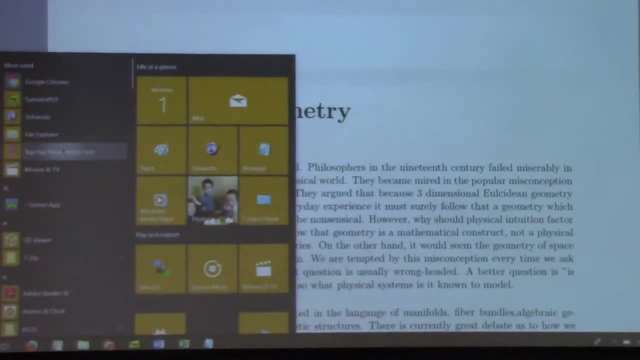 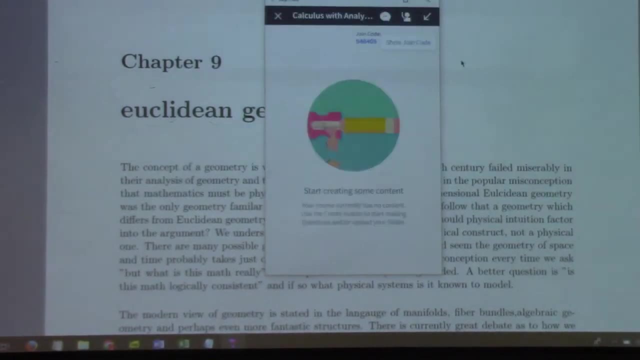 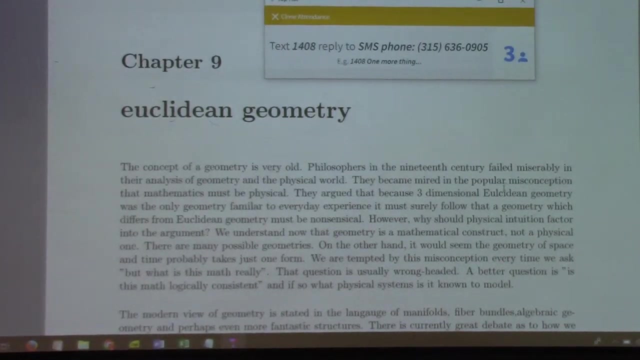 that I have thrown under the bus and not talked about so far. today you can do it. you don't want to 10 calculus to write, you'd rather take calculus to you, I think, in some senses get some sense, calculus two's harder in this course. but anyway, for 1408 is the magic number, 1408. 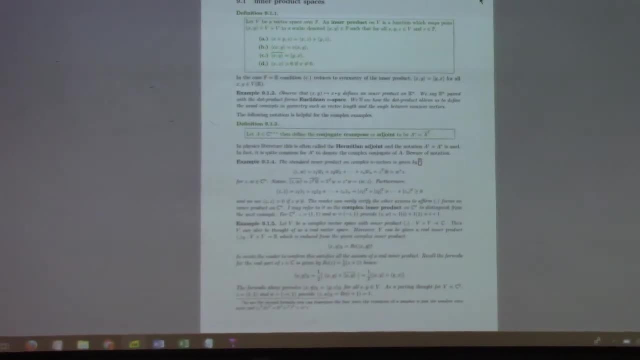 now, the thing I haven't defined yet- and I should have- well, I'll look at it on the projector- is angle. we can define the angle between vectors, all right, and there are two different notions of angle to define: complex versus real. now for a real vector space. you already got it for a real vector space. whoa, it's easy. 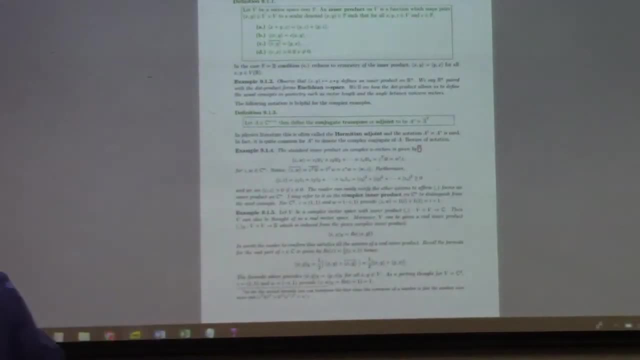 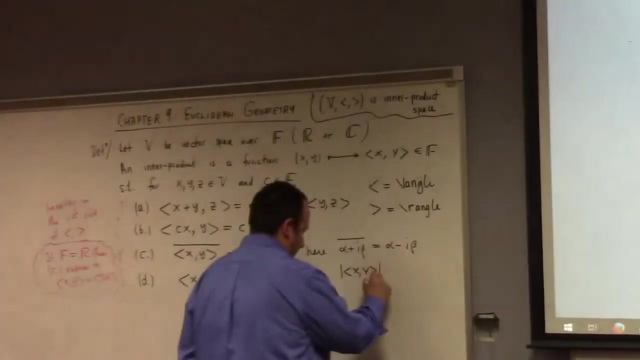 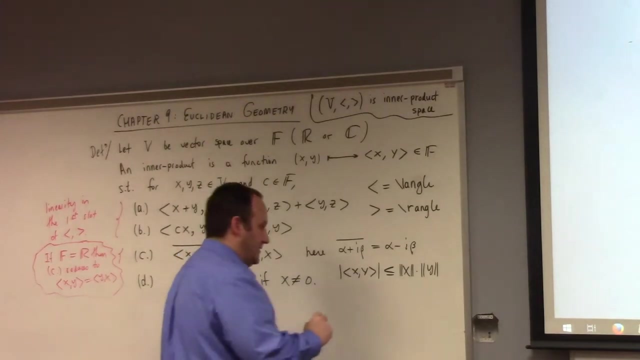 enough. so the thing is we have that the, the modulus of XY is less than or equal to the norm of X times the norm of X times the norm of X times the norm of X. okay, and so what that says is that, if we look at the EPSA value or more generally, 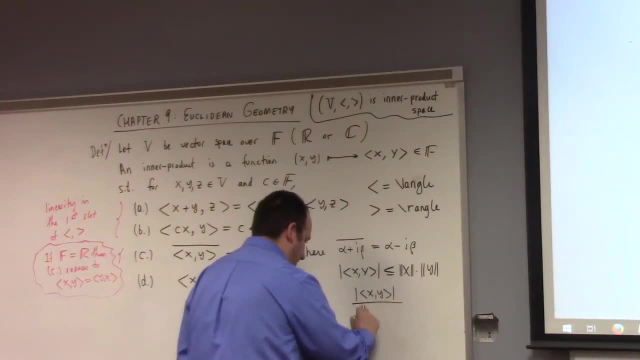 the complex length of the inner product X and Y divided by the norm of X times the norm of Y, that's that's less than or equal to 1. this is always true, but in the case that we're working in the real field, we can say: minus 1 is less than. 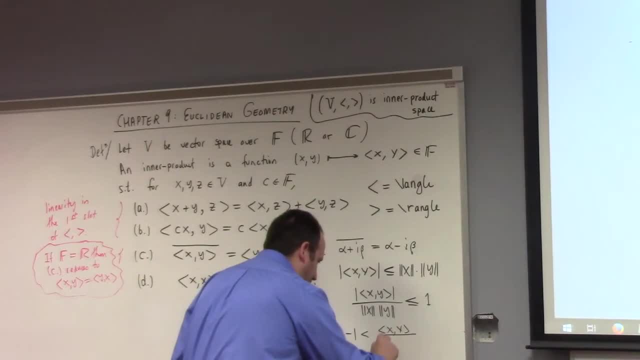 the EPSA value- they see me- minus 1 is less than the inner product of x and y. norm of x times the norm of y is less than, less than or equal to 1. so this is both of these, all this whole discussion here. I'm assuming x and y are 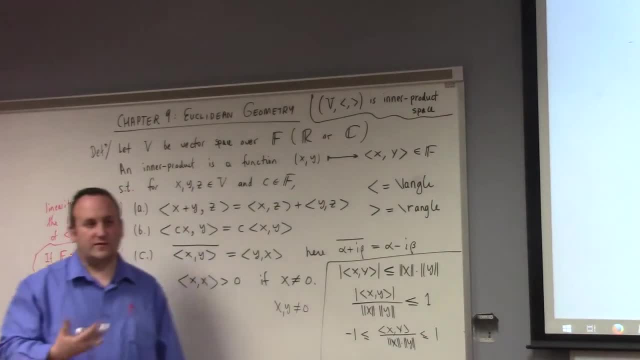 not equal to 0 effects and y are not equal to 0, we can use the Cauchy- Cauchy-Schwartz inequality to motivate defining the angle between the vectors. all right, and one of the things I neglected to say here so far, and I 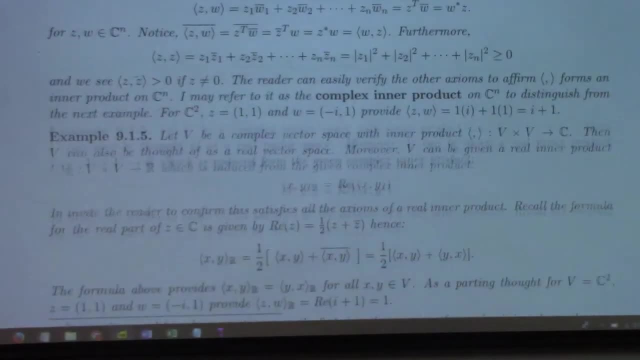 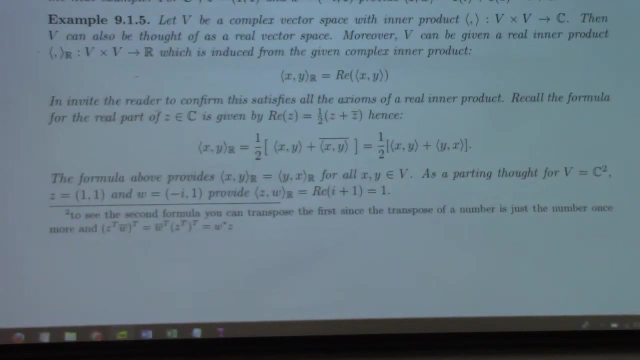 probably should say a word about is that, even for a complex vector, if you have a complex inner product space, there is an underlying: every complex vector space is also a real vector space. right, because you can just restrict the scalars to be reals and so like, if I take a real vector space and I take a real vector space. 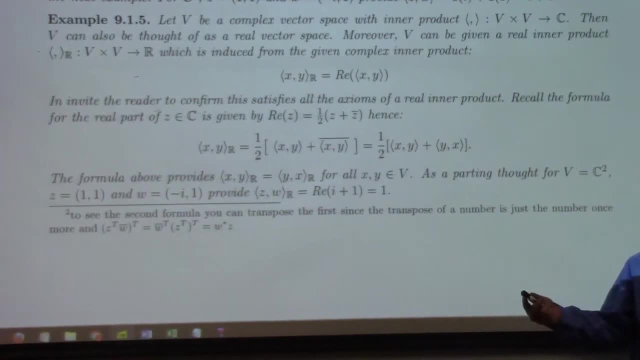 and I take c2. it's a two-dimensional complex vector space, right, but it's also a four-dimensional real vector space, so I can always take a complex vector space and look at it as a real vector space. I can also take a complex inner product space, like a complex vector space which has an inner product in that sense, and I 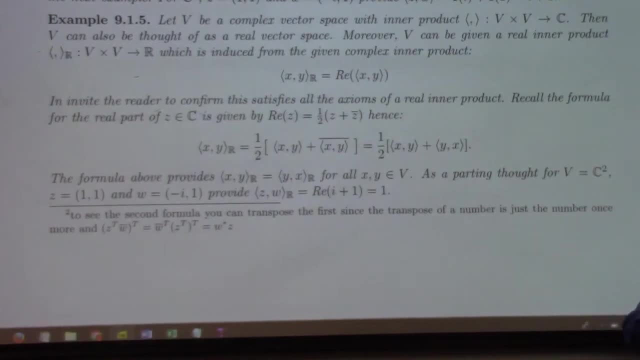 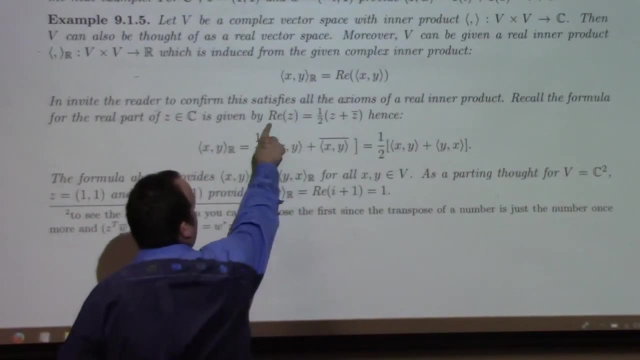 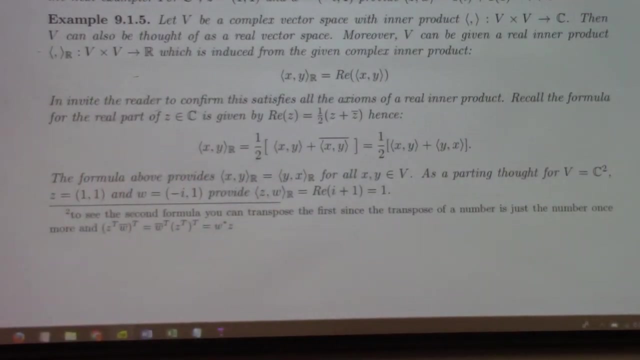 can construct a corresponding real inner product from that complex inner product like this. so the, the real inner, the underlying real inner product, it's just defined to be the real part of the complex inner product and you can, you can work out that it. um, it works out nicely actually. here's, for example: if i had z equals to 1, 1. 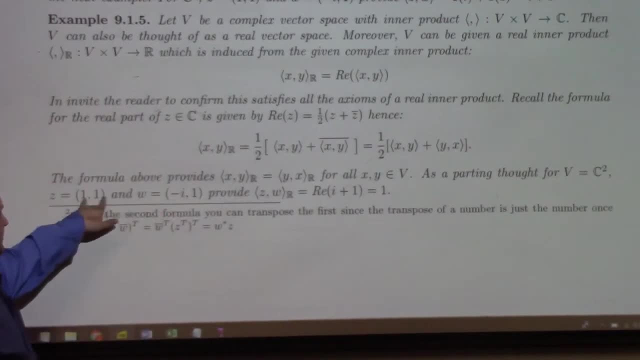 and w equals to minus i 1, then the complex inner product of this, and that is 1 times w the conjugate of that which is i, so that gives me i plus 1. i plus 1 is the complex inner product of these two vectors. the corresponding real inner product is just the real part of this, which is 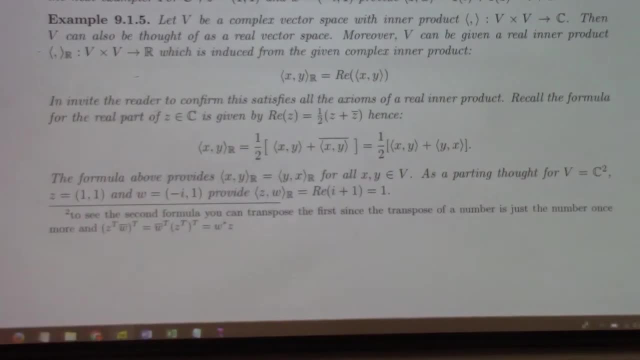 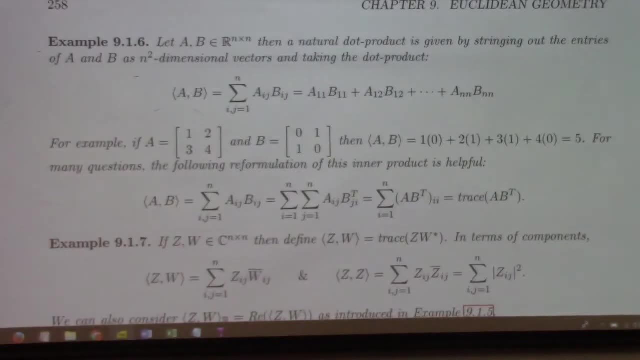 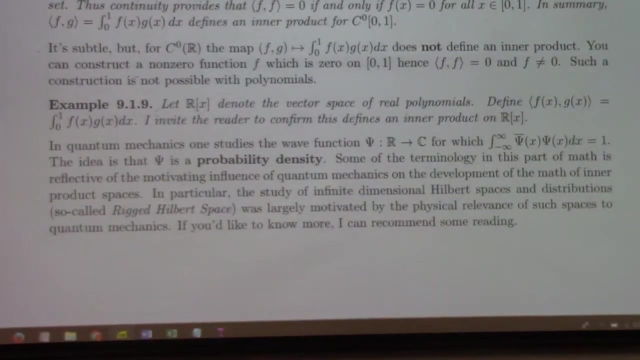 just one. so they're just. they're different concepts, but they're both available for a complex vector space. so we just talked about that example and that example. there's that example. great, you could just as well define the inner product of the complex inner product on all polynomials by the integral from 0 to 1, of f, of x, g, of x, dx. 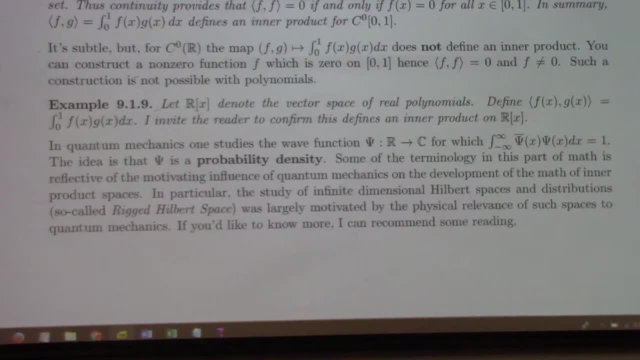 it's still the case that if you know, if you have a polynomial and the integral of the square of that polynomial from 0 to 1 is 0, that forces the whole polynomial to be 0. but if you thought about arbitrary continuous functions on the reals it wouldn't work because 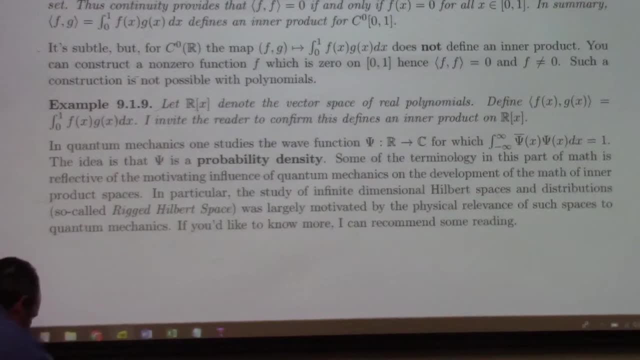 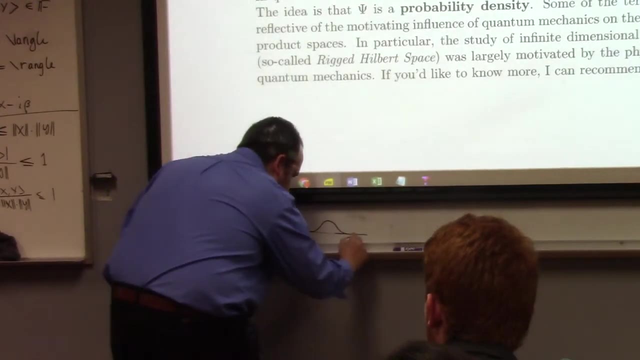 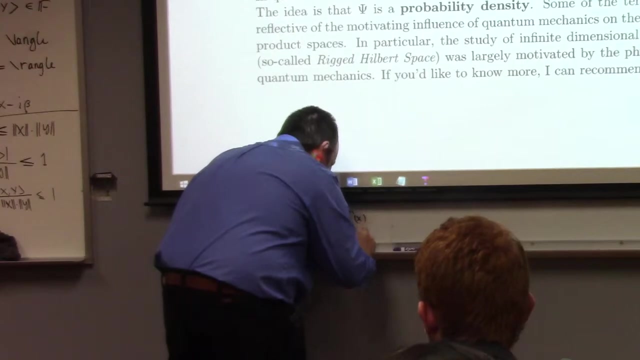 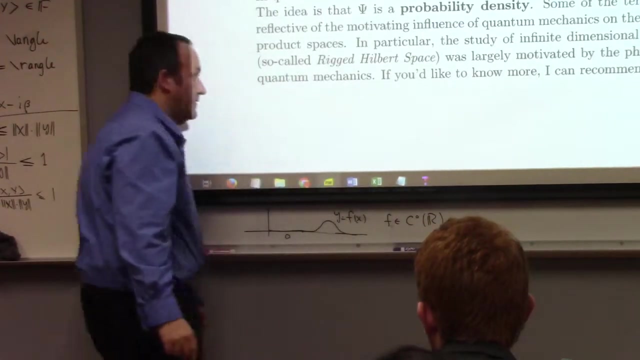 arbitrary continuous functions on the reals. you could have the situation like this: it's 0, like that, but then over here you got some hump right and if this is what the graph of f, of x, looks like- you know, for f, some continuous function on the reals, then that means, if i tried to 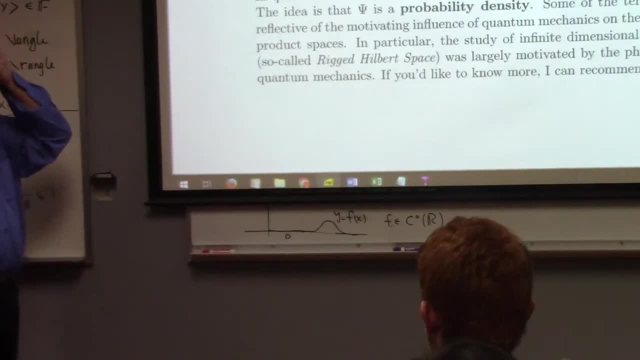 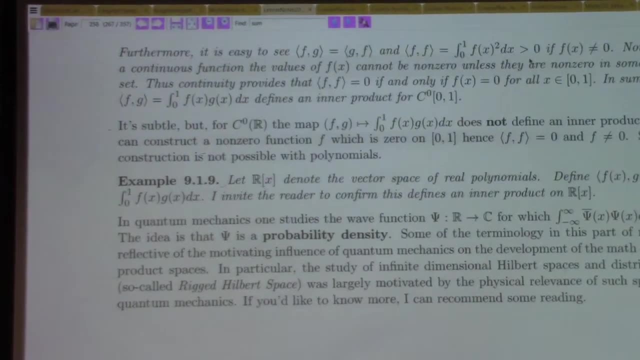 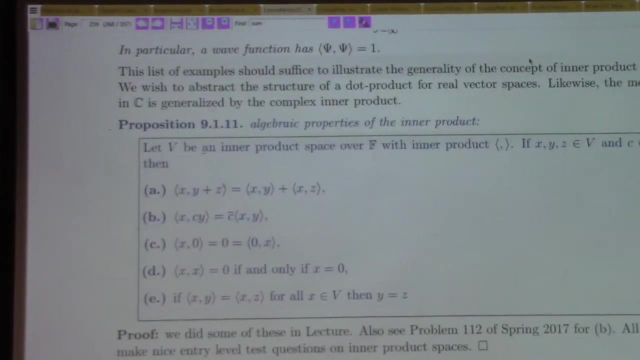 define the inner product just integrating from 0 to 1 continuous functions? that wouldn't work right. i think you have a homework problem which is basically begging this question, so i'm going to go on, though, because we have other things here, so these are derived things you can derive from the axioms that, for example, you can prove that you also have 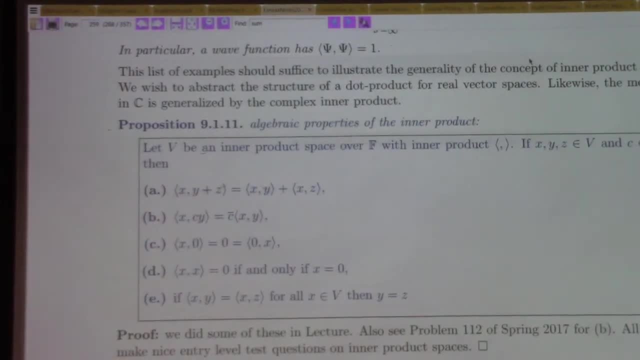 additivity in the other. so if you have a, b, c, d are true, we can get. these are our direct consequences. the proof is down here. um, well, actually it's not, but you can prove that the we have additivity in the second slot if you pull a constant out of the second and then you get things like. these are like: 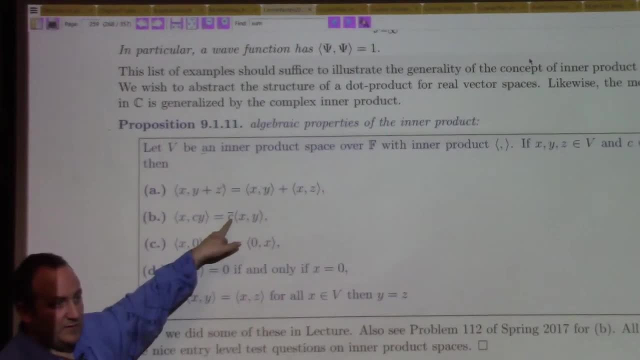 component, you get complex conjugate. generally speaking, for a real inner product, you can just pull numbers out. you know, like the dot product, if you have a scalar multiple either of the vector multiplying either the vectors, your dot product and you can pull that number out. right. but if we're 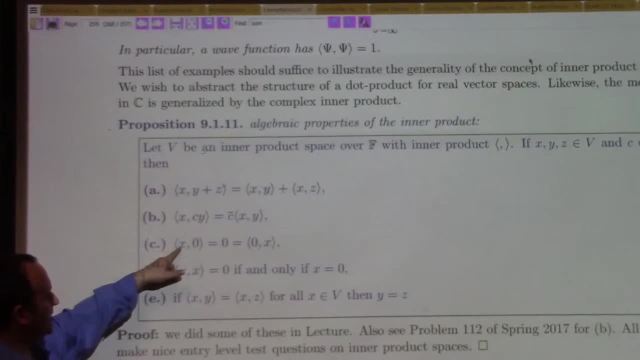 in the complex case we have to pull out a conjugate there. inner product of any vector with a zero vector is zero. this says what this is. zero is orthogonal to everything, yeah, every, everything. and and finally, this is something I've been checking on, right, because this is one. 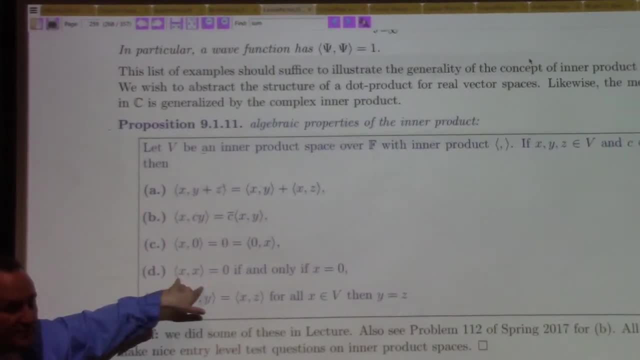 of the things I can tell whether or not some things in inner product. if the inner product of X when the X is 0 for some X not equal to zero, then game over, it's not an inner product, because this is something that's true for inner products. and then as far as this kind, 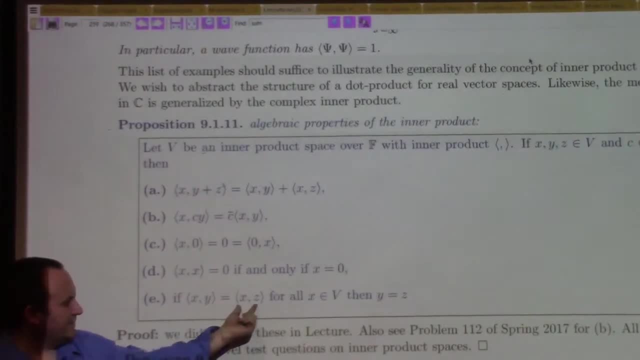 of cancellation property. if you have X dot X, X inner product Y is inter equal to X inner product Z, and if that's true for all X, then that imp always implies y equals to Z. it's not enough to know that it's true for 1x, can you guys? 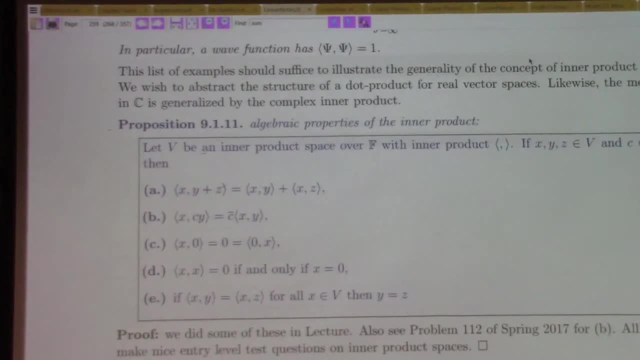 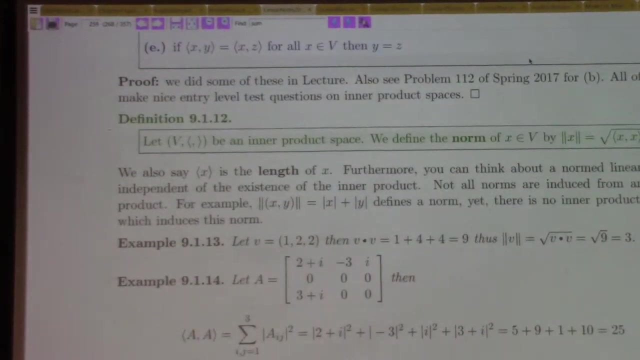 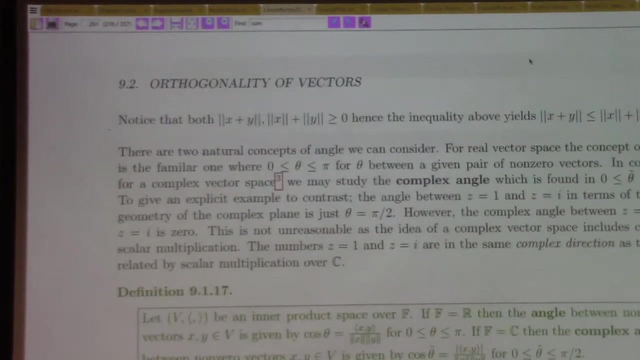 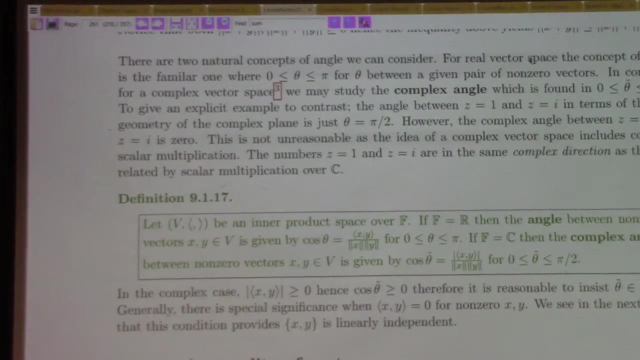 think about something in between for 1x and for all, for all, for all X. that would still give you truth there in a vector space. well, the answer to that is: if you did it, if you had equality for a basis, that would be enough. you could prove that that this is, it's enough. so, anyway, this: 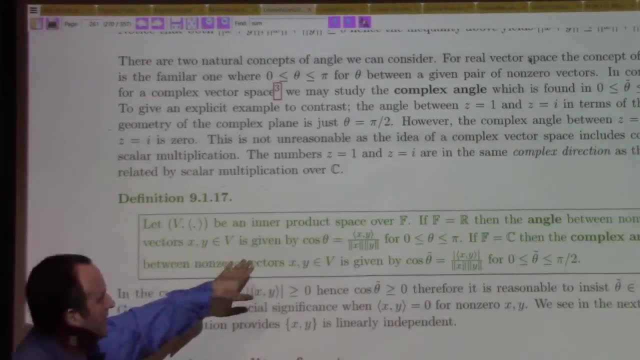 is what I was trying to get to. for a real in a product space, the angle between two vectors is defined implicitly by cosine of theta is interproduct of x and y over this. that gives you an angle between 0 and n- pi. but if we're dealing with a complex in a product space, we can also define the.